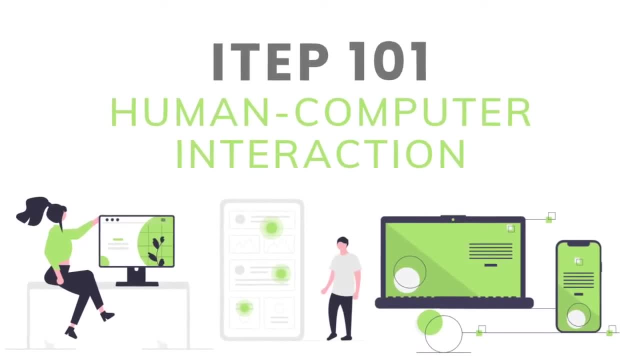 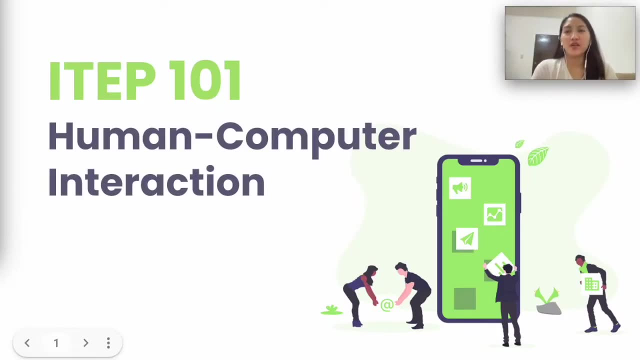 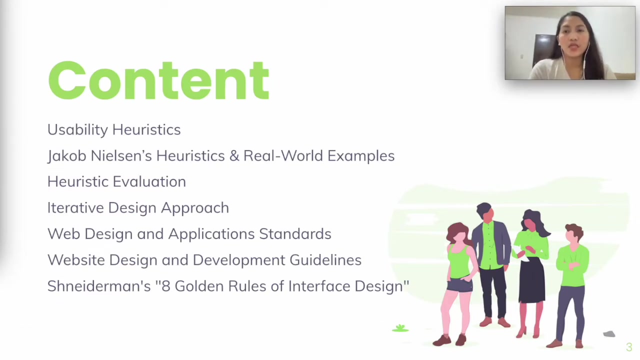 Good day everyone. This is video lesson in ITEP 101, or Human to Computer Interaction. This video lesson will cover the first part of Module 2, which is the lesson entitled Principles of Software Usability. The topics here include Usability, Heuristics, Jacob Nielsen's Heuristics and Real-World Examples- Heuristic Evaluation. 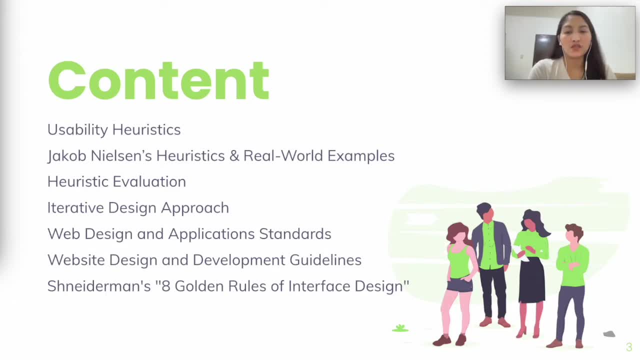 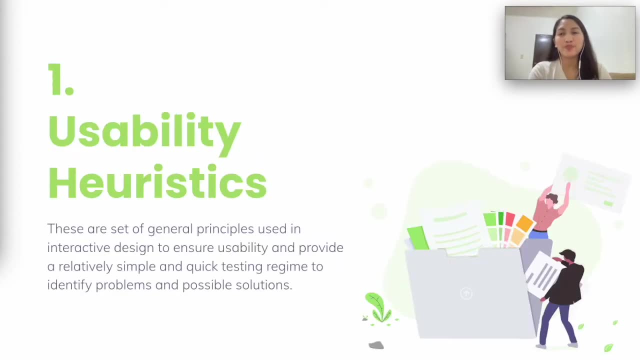 Iterative Design Approach, Web Design and Application Standards, Website Design and Development Guidelines and Schneiderman's Eight Golden Rules of Interface Design. Now let's proceed to the first topic: the Usability Heuristics. When you say heuristics, these are a set of general principles used in interface design. 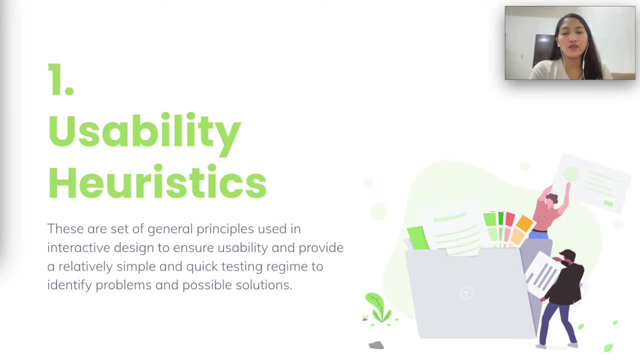 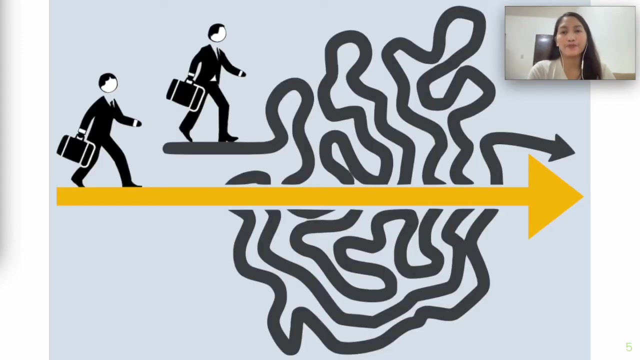 Heuristics is an interactive design to ensure usability and provide a relatively simple and quick testing regime to identify problems and possible solutions. The reason why we use heuristics is to ensure usability when you design the user interface. When you say heuristics, the term heuristics means mental shortcuts that can facilitate problem solving and probability judgments. 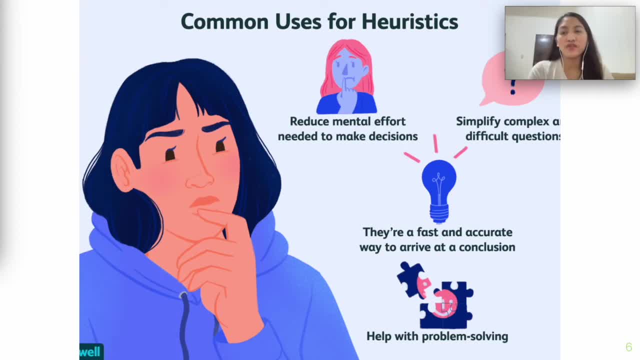 These strategies are generalizations or rule of thumb to reduce cognitive load and can be effective for making immediate judgments. However, they often result in irrational or inaccurate conclusions sometimes, But moreover, heuristics is very helpful when you want general principles to guide you in the design of a user interface. 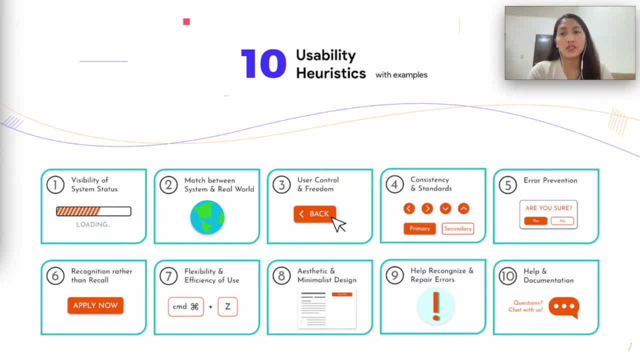 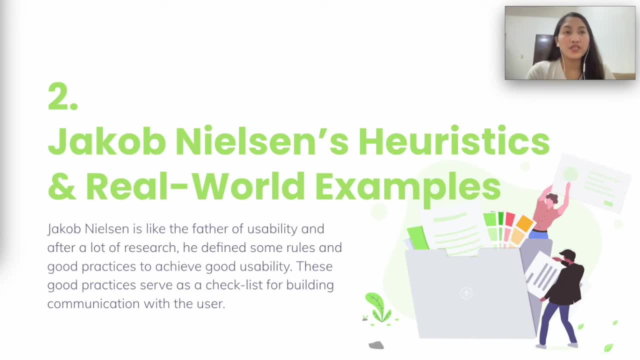 They are called heuristics because they are broad rules of thought. They are not specific usability guidelines. Now let's discuss one of the heuristics that are available, And the most common is this: the Jacob Nielsen's Heuristics. So who is Jacob Nielsen? 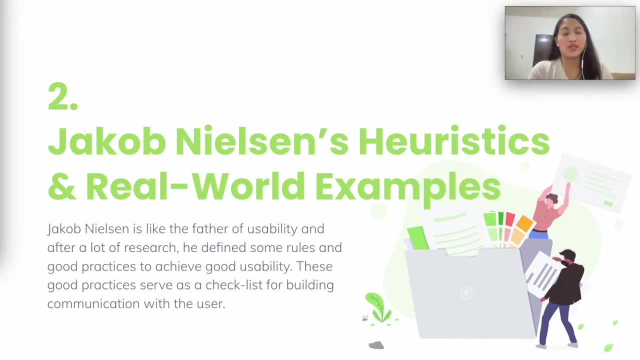 Jacob Nielsen. he is like the father of usability And after a lot of research he defined some rules and good practices to achieve good usability. These good practices serve as a checklist for building communication skills. For example, if you want to learn how to use Heuristics, you need to know how to use Heuristics. 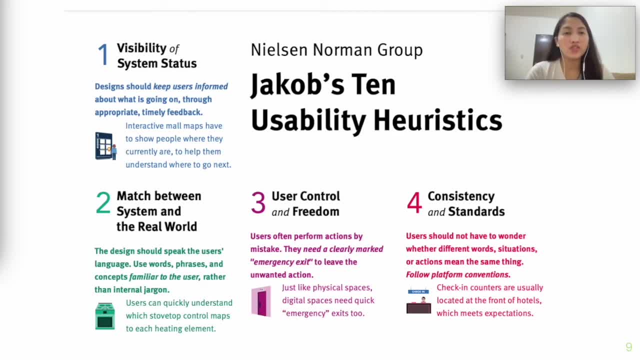 So this is just an overview of Jacob's 10 usability heuristics. So we have here the visibility of system status as the first. Second match between the system and the real world. Third, user control and freedom. Fourth, consistency and standards. 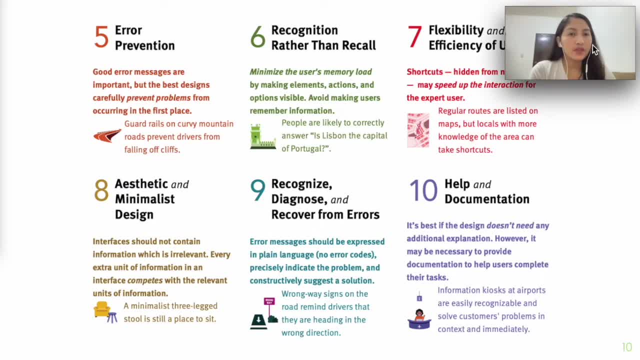 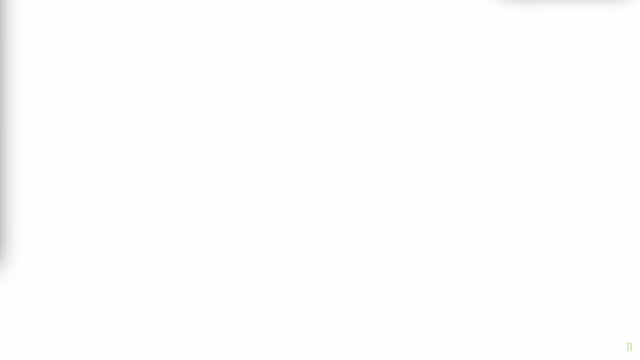 Fifth, error prevention. Sixth, recognition rather than recall. Seventh, flexibility and efficiency of use. Eighth, aesthetic and minimalist design. Nine, recognize, diagnose and recover from errors. And the tenth is help and documentation. So now let's discuss each heuristic. 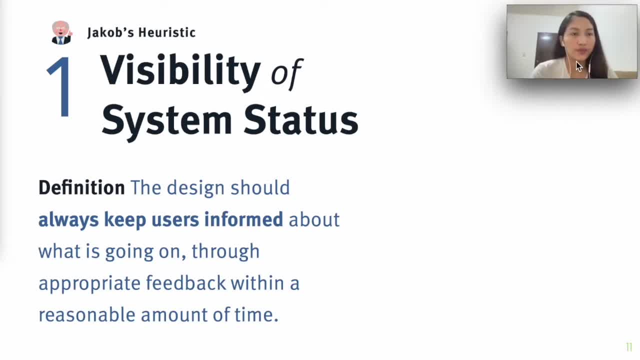 The first one is the visibility of system status. So, as defined here, the design should always keep the users informed about what's going on through appropriate feedback within a reasonable amount of time. So let me discuss with you some tips for you to be able to apply this first heuristic. 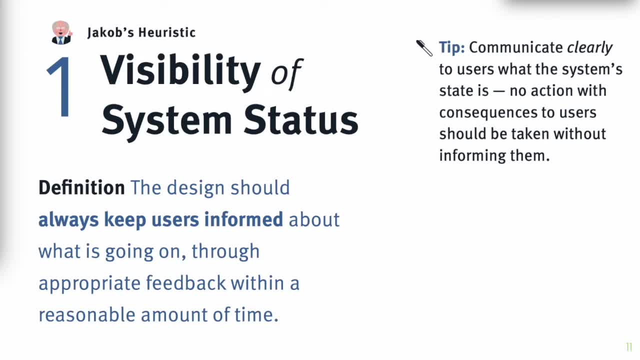 So the first tip: communicate clearly to users what the system state is. No action with consequences to users should be taken without informing them. Second, you have to present feedback to the user as quickly as possible. And third, you have to build trust through open and continuous communication. 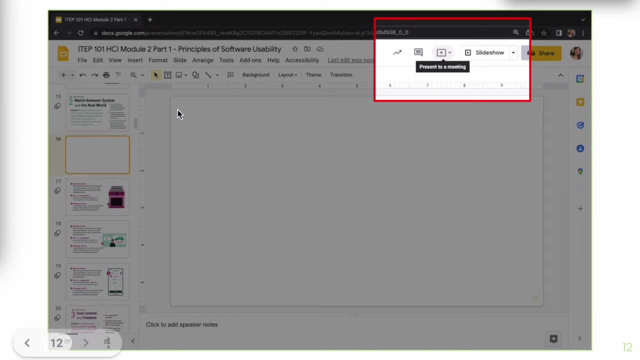 So as an example, I have used Google Slides, for example, for each heuristic. So for the application of the first heuristic in Google Slides, whenever you mouse hover a command or a button or a control and information about that specific command or control button is being displayed, just like this one. 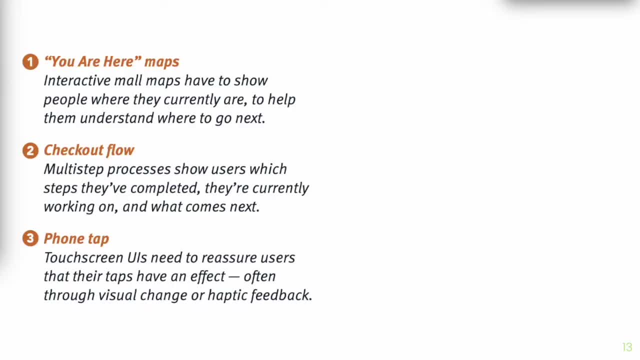 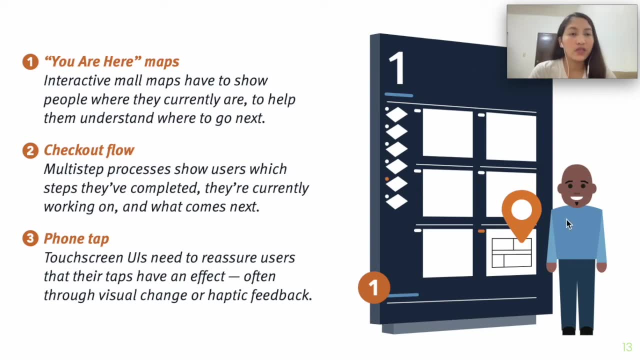 So let me show you another example. Let us walk through this quickly. So the first one is the You Are Here maps. So I know you are all familiar with this kind of maps. So the You Are Here maps are interactive mall maps that shows people where they currently are. 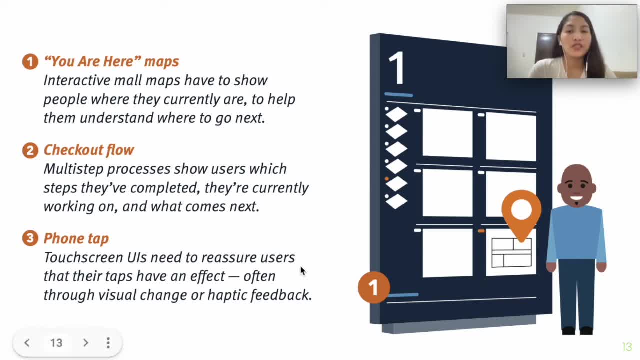 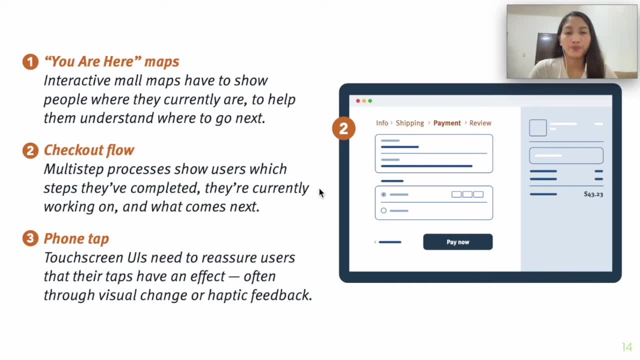 to help them understand where to go next. Another is the checkout flow. So in the checkout flow, the user is being shown a multi-step processes in order for them to know the steps that they have completed, the steps that they are currently working on and what comes next. 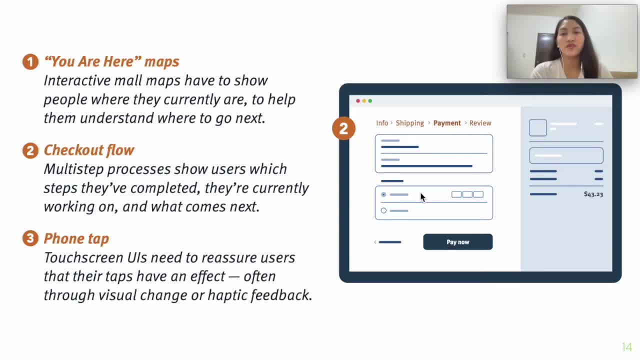 So the next application or the real-world example of this heuristic, the first heuristic is the phone tap. In the phone tap the touchscreen UIs need to reassure the user that they are in the right place. In the phone tap the touchscreen UIs need to reassure the user that they are in the right place. 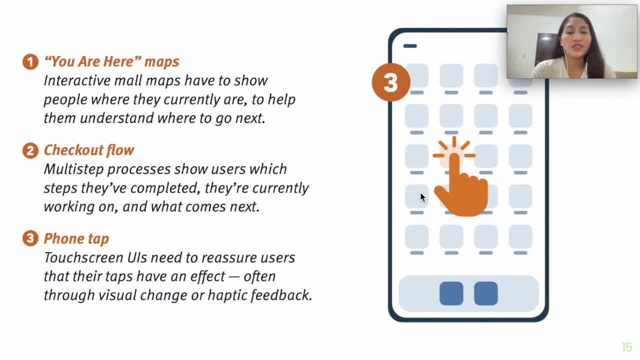 In the phone tap the touchscreen. UIs need to reassure the user that they are in the right place. When the user taps the phone, it has an effect. It could either be a visual change, change in the color or haptic feedback. 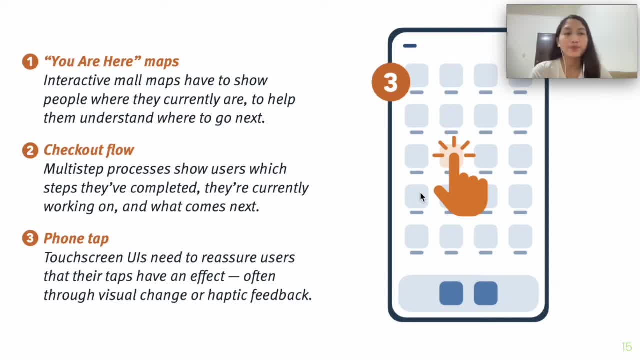 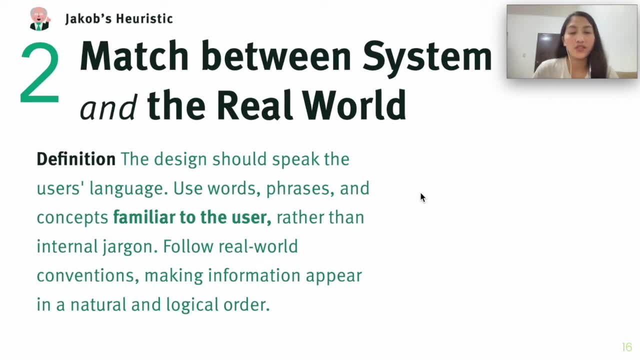 or you can feel a slight vibration when you touch the phone. So that's the first heuristic: visibility of system status. Now let's proceed to the second heuristic, the match between system and the real world. So in the second heuristic, the design should speak the user's language. 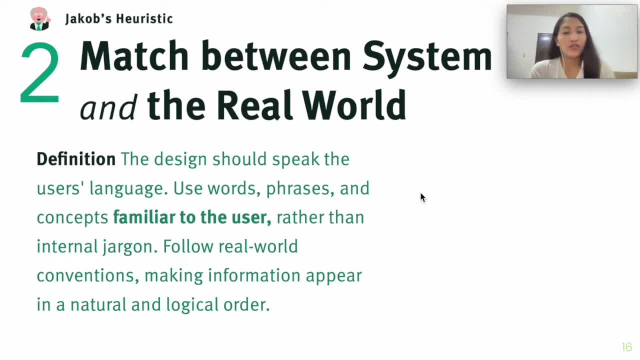 So in the second heuristic, the design should speak the user's language. So in the second heuristic, the design should speak the user's language. So what does that mean? You need to use words, phrases and concepts that are familiar to the users. 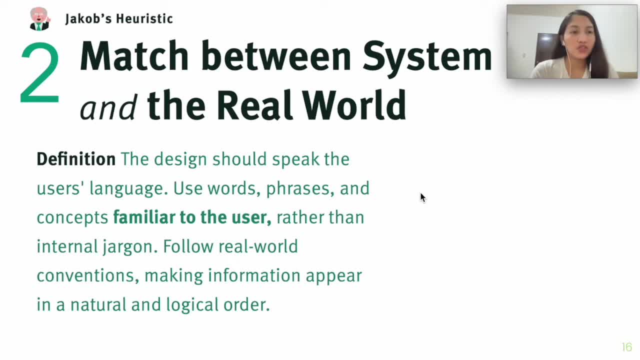 Rather than internal jargon. When you say internal jargon, these are the words that only a programmer knows. You should use the terms, words, phrases and concepts that are familiar to your target users. So how will you do that? 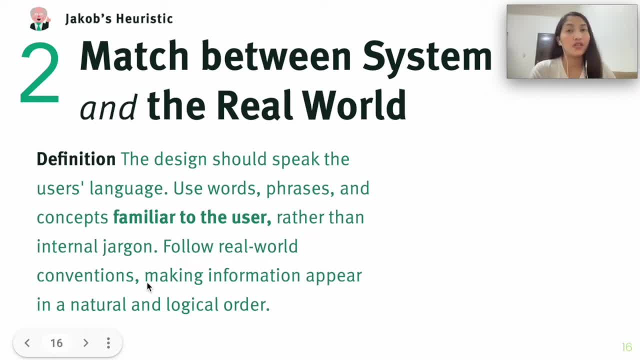 Just follow the real-world conventions Making information appear in a natural and logical order. So here are some tips to apply the second heuristic, the match between system and the real world. First, ensure users can understand meaning without having to go look up a word's definition. 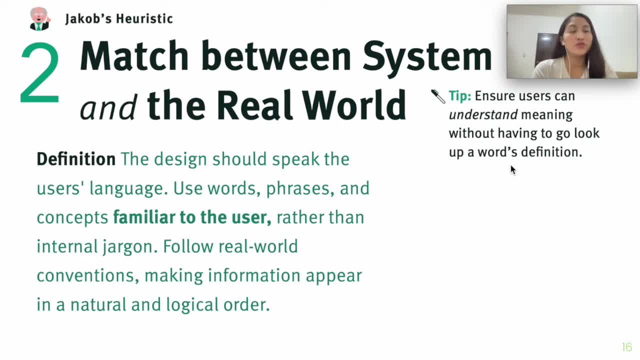 So kapag naman ginamit mo yung words, yung terms, yung phrases at yung concepts na ginagamit talaga ng target users, they don't have to look to the definition of that word. 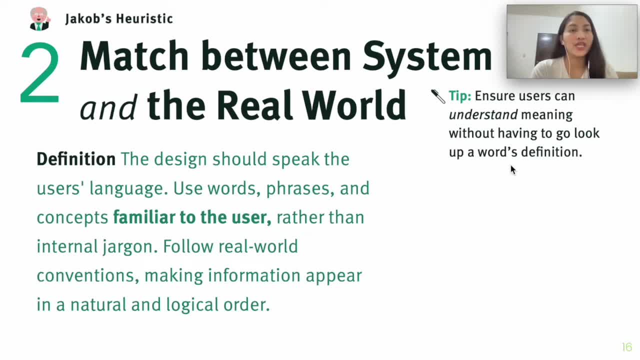 Para magamit nila yung command or yung function na inilagay mo doon sa system. Pangalawa, never assume your understanding of words or concepts will match those of your users Because, again, you are the programmer, you are the designer, but you have to adapt or adjust to the need of your users. 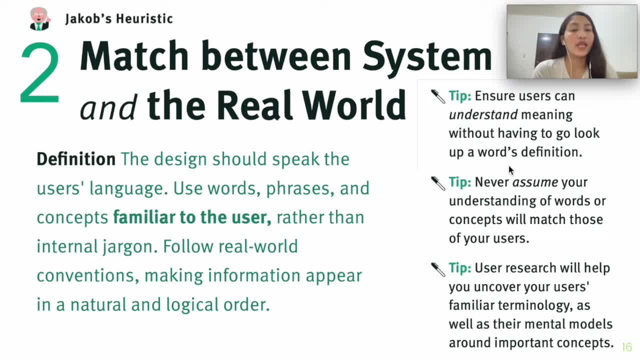 And the third tip- ito yung sinasabi ko kanina: user research will help you uncover your users' familiar terminology. So gather This information data, or this important data, Okay. aside from that, the terminologies that they are using kailangan i-uncover mo din yung mental models around important concepts ng target users mo. 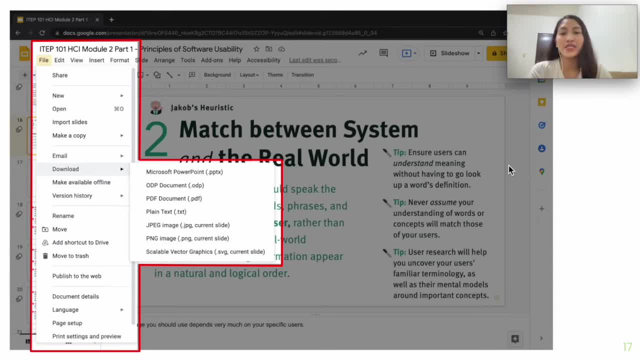 Okay, so this is an example again sa Google Slides. If I want to download the file, I just have to go through the in the main menu. familiar ako na nasa file siya. hindi sa edit, hindi sa view, hindi sa insert. 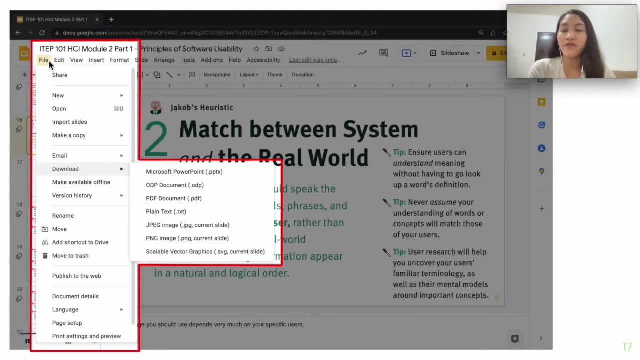 Because the users are familiar with the download being in the file menu, then they have included that command or control here in the file menu where you can download the slides in different formats. So ayan, kita din nila yung file extension for the different downloads. 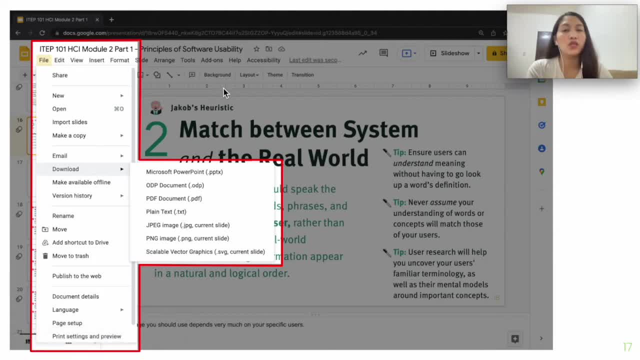 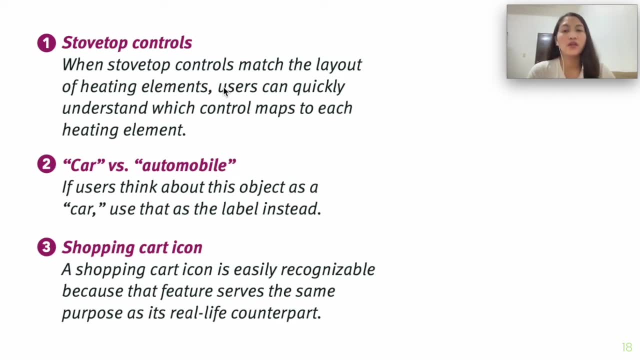 Available If you want to download a file, a Google Slides file. So another example or examples: we have the stove top controls. So sa stove top controls naman, yung controls, it should match the heating elements or the layout of the heating elements. 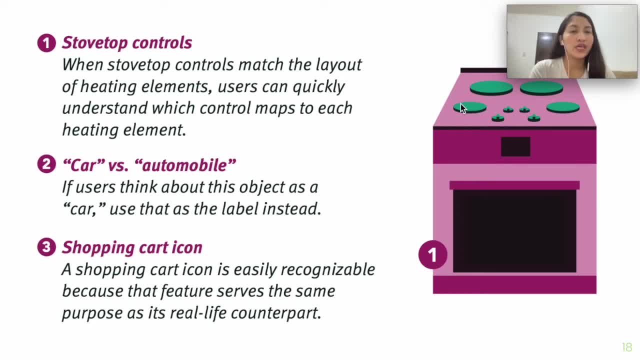 So in this example, if you want to turn on this heating element, you just have to turn this knob, Okay, And yeah, the other knobs respective of the position or the layout of the heating elements. so again, there should be a match between the system and the real world. so the second is: there are countries. 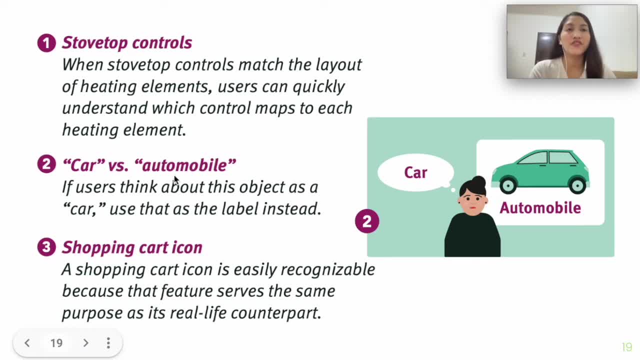 or nationalities that uses different terminologies for the same word with the same meaning, for the same for words that has the same meaning. an example would be car versus automobile. so if the users think about this object as car, then use car as the label instead of automobile. 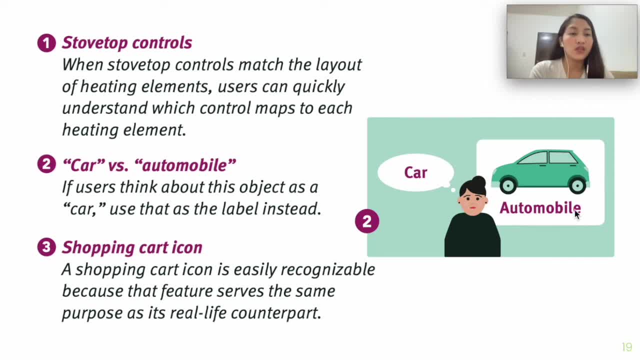 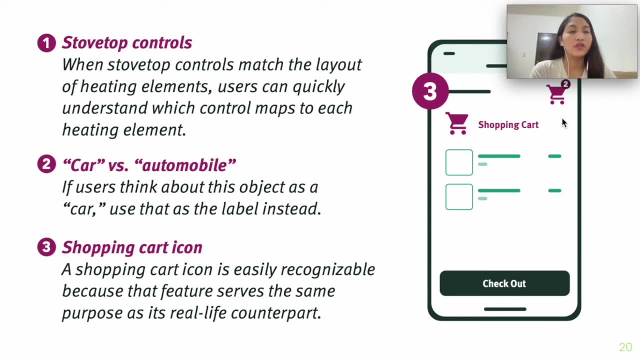 there are countries that uses automobile. they are familiar with the car, with the term automobile instead of the term car, so use that instead. and then the third one, the shopping cart icon. this is easily recognizable. this means that you are adding something in your cart to shop, or. 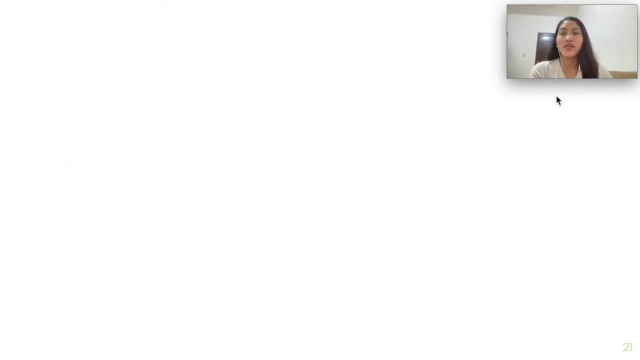 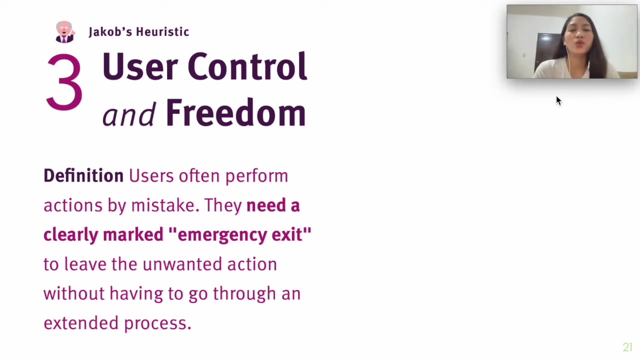 to buy. okay, so that's for our second um, second juristic, the match between the system and the real world. now let's proceed to the third. the third is the user control and freedom. so minsan yung mga users, they perform actions by mistake. so if that is the case, they need a clearly 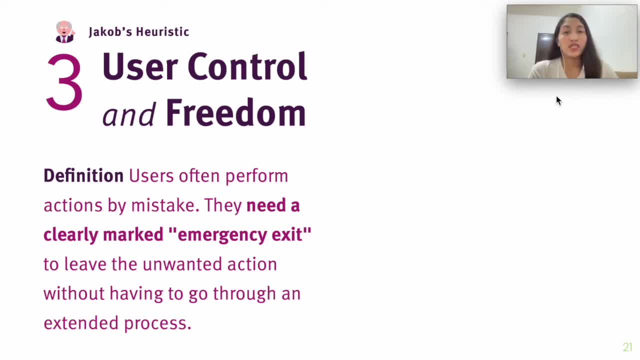 marked emergency exit to leave the unwanted action without having to go through an extended process. so to do this, syempre dapat iya assume natin na mag make ng mistake yung users natin. you have to support, undo and redo. this is very helpful, especially sa mga video editing image. 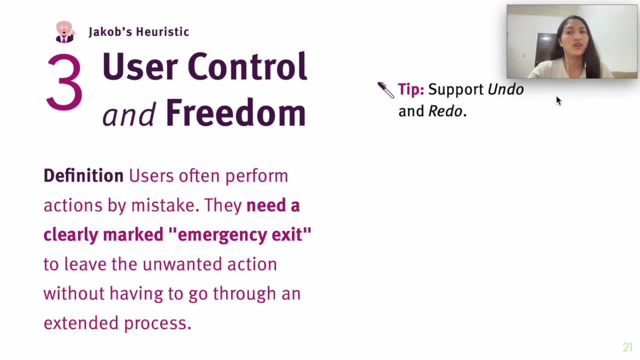 editing apps kasi pwedeng ayaw nila nung effects na yon, so they you have to give them the option to either undo or redo actions. second, show a clear way to exit the current interaction. so halimbawa, um they have created a mistake, um uh na hindi nila intended, kailangan meron kang clear way to exit. 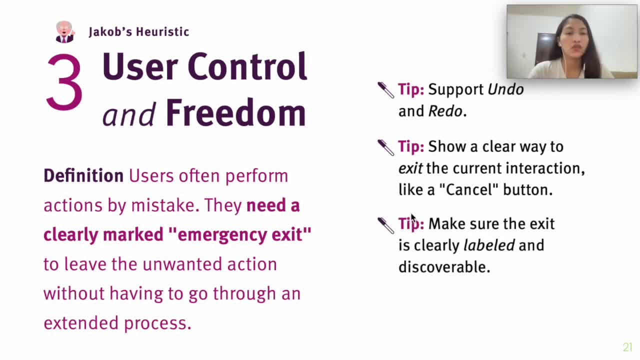 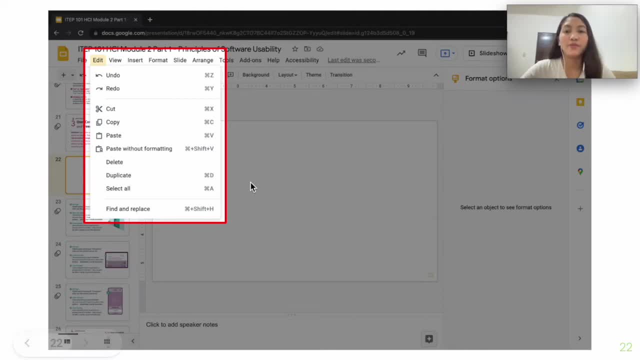 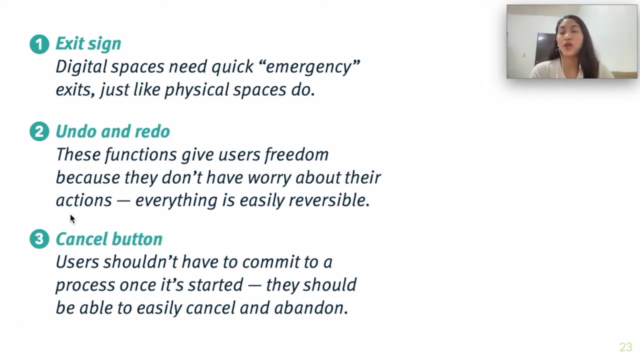 like a cancel button. and then the third tip is to make sure that the exit is is clearly labeled and discoverable. okay, so this is an example. again in the google slides, undo and redo actions, um are being supported. so next examples are: um for this juristic is the exit sign. okay, so kung ang mga physical spaces 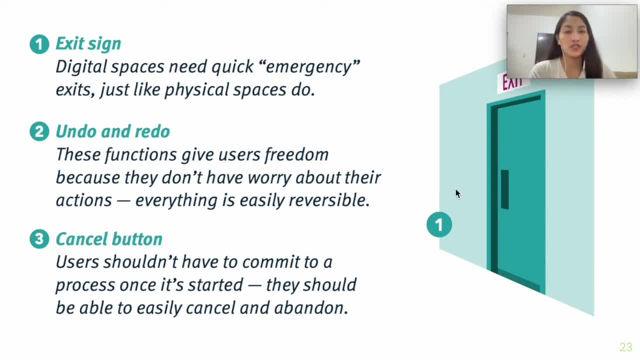 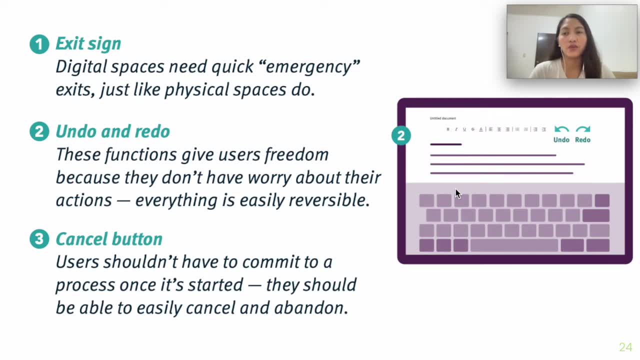 merong exit sign. ganun din dapat yung mga digital spaces dapat meron ding emergency exits. so the second, again, as uh we have uh presented or i have presented a while ago, is the undo and redo actions. um you have to let your users um not worry about their actions, because everything is easily. 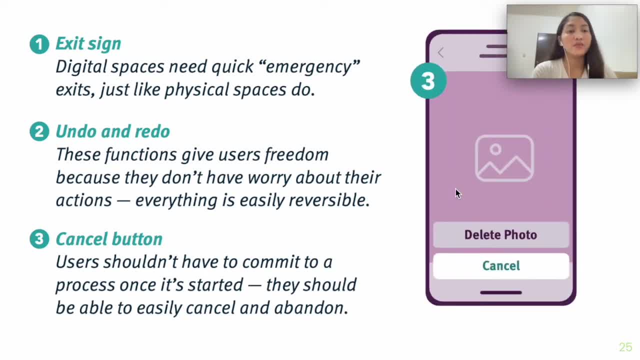 reversible. and the third one is the cancel button. uh, whenever a user wants to have an action, uh that may have an impact on your um, on your users, then if, if that is an accident, then, um, you have to show them. uh, an easy way out, for an example, would be deleting a photo. most probably they don't want to delete that photo. 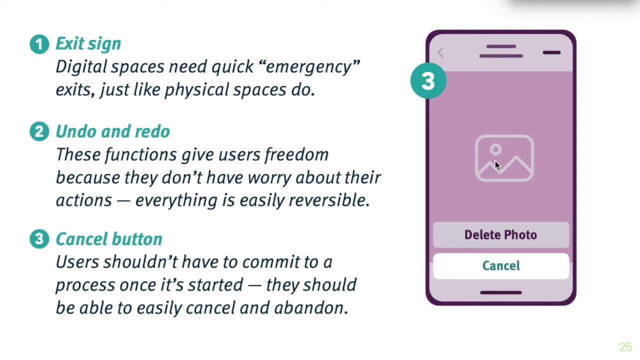 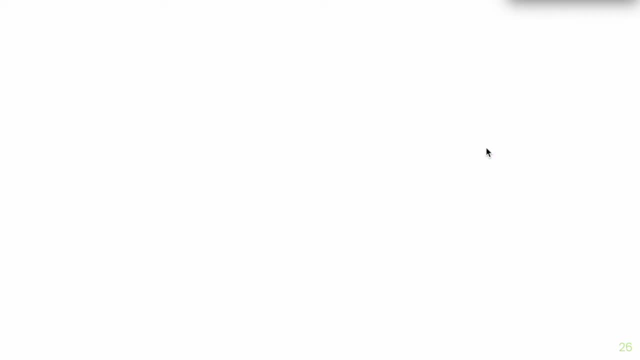 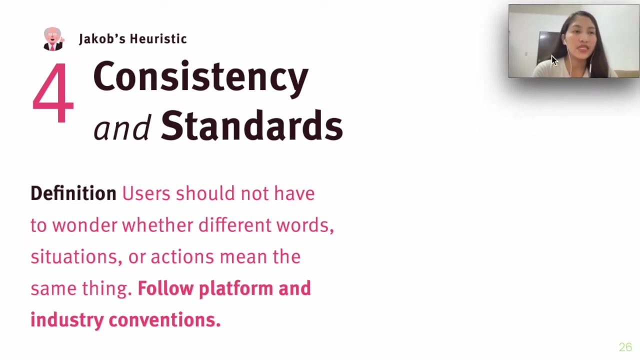 and yet, um, they have. they have done an action by mistake, so you have to give them an option. even if it's not an accident, even if that is intentional, uh, still give them this um option, okay. so the first, the fourth um, juristic, is the consistency, and 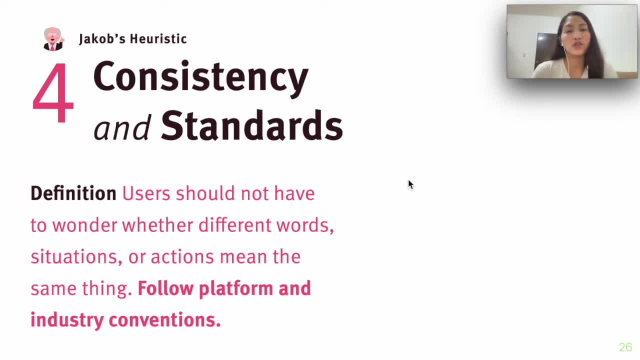 standards, so your user indicators should not have to wonder whether words, situations or actions mean the same thing. so meron tv platform and industry conventions. so you have here um some tips. the first step is to improve learnability by maintaining both types of consistency: internal and external. 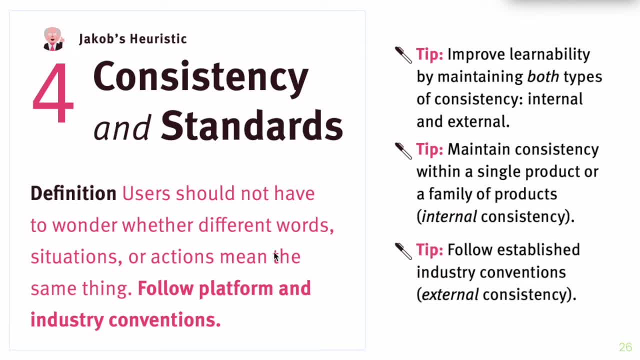 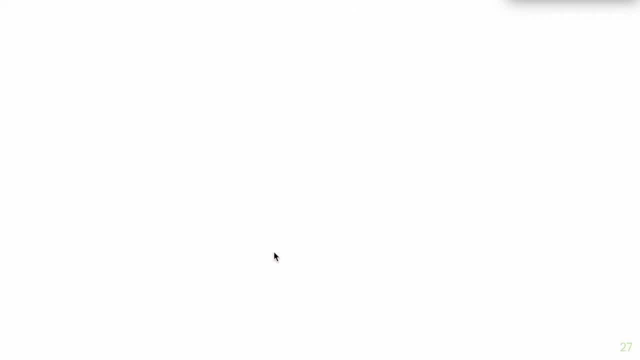 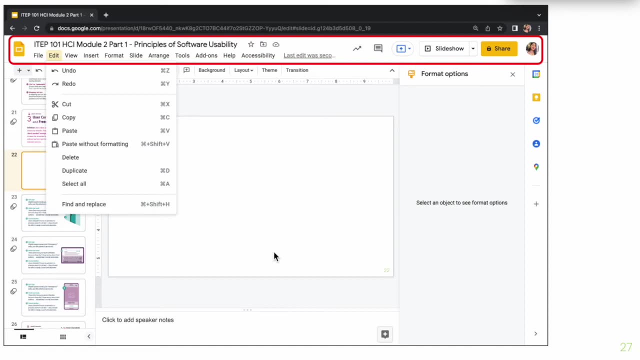 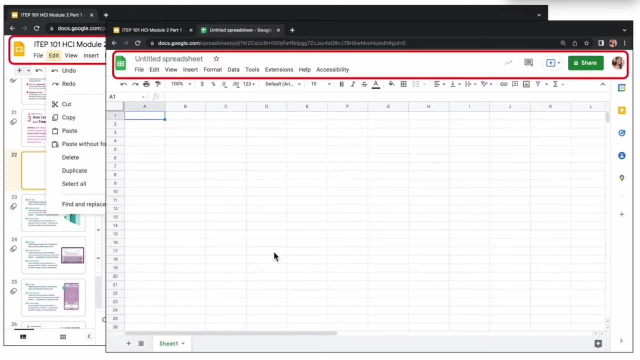 so next, uh, next, Next tip is the follow established industry conventions or the external consistency. So we have here again example would be the Google apps, Google documentation apps. I have here for the Google slides and the Google sheets. you know the look and feel. 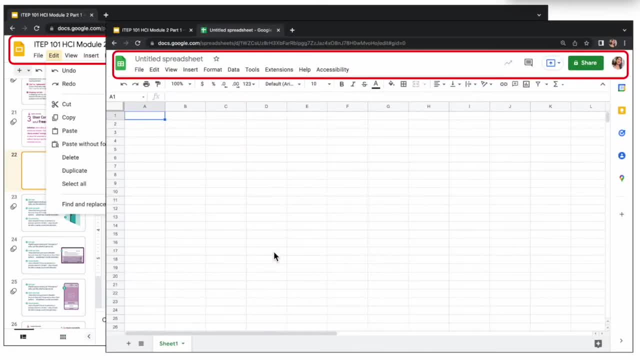 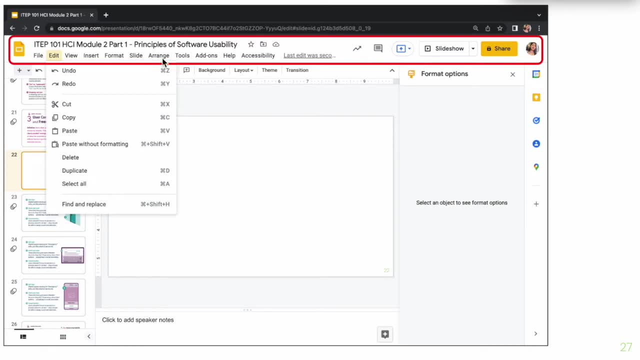 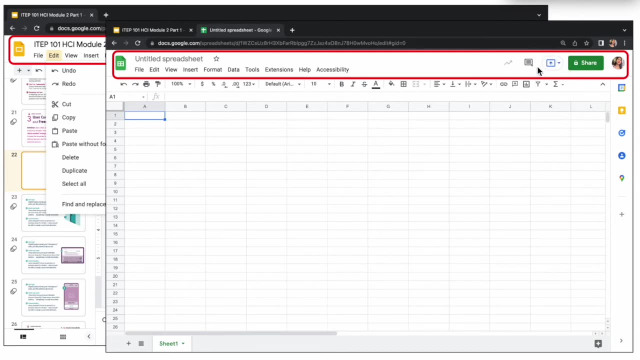 of the main control menu on top of the Google document processing apps are the same across platforms, such as file edit, view, insert, format and others, And even the share button and the presentation or the other menus. you have this. you are. 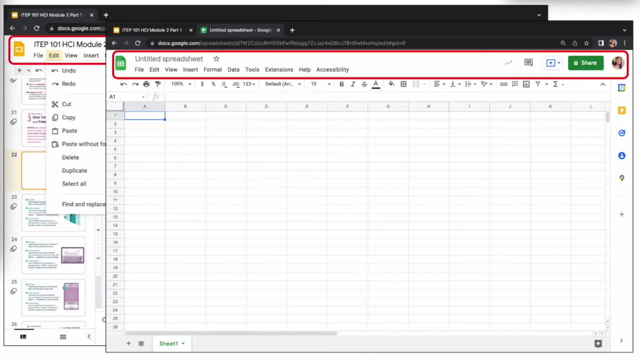 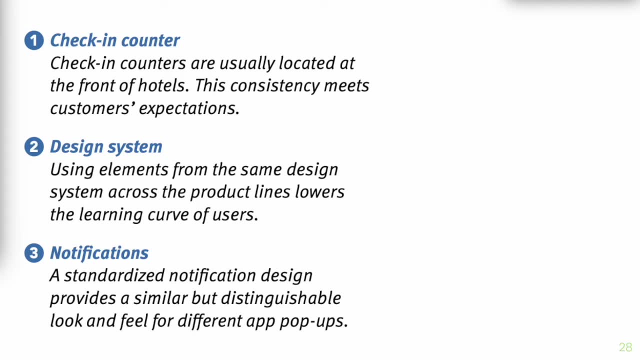 familiar with the look and feel. if you will jump from one platform to another, So another or real world examples are check in counter In front of the hotels, as well as when you adopt this in an information system. your user should be. you know you have to follow the conventions of your users. 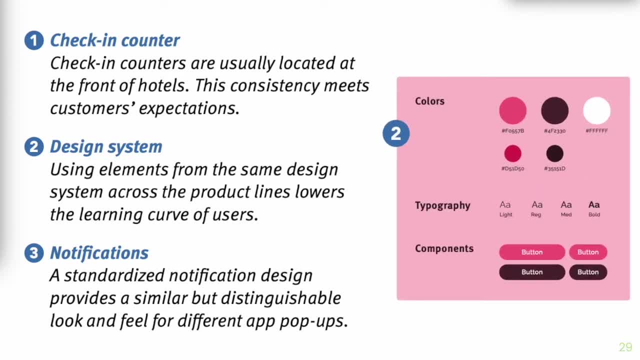 And then in the design system you have to use the elements from the same design system across the product lines. It lowers the learning curve of the users. So Just like the shape of the button, the color of the font, the color of the background. 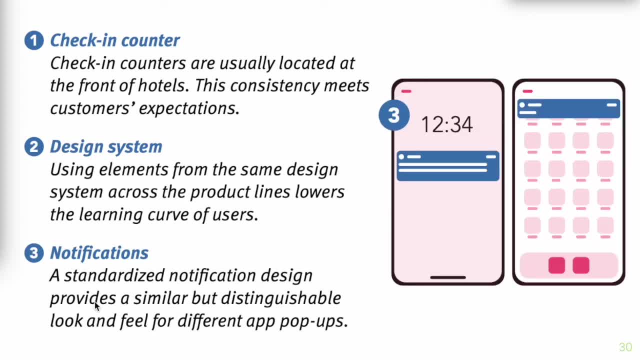 etc. And then the notifications, The standardized notifications are. I know you are very familiar with this application of this heuristics. Okay, So the color of the notifications, the feel of the notifications, probably also the font style and the font color and the font size are the same. 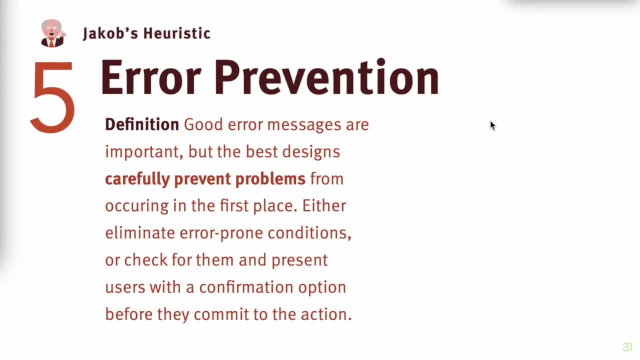 So the fifth heuristic is the error prevention. So it's like it's like the same with the previous heuristic, But a difference is the good error messages are important, But the best design carefully prevent problems. So this is the difference with the sister. 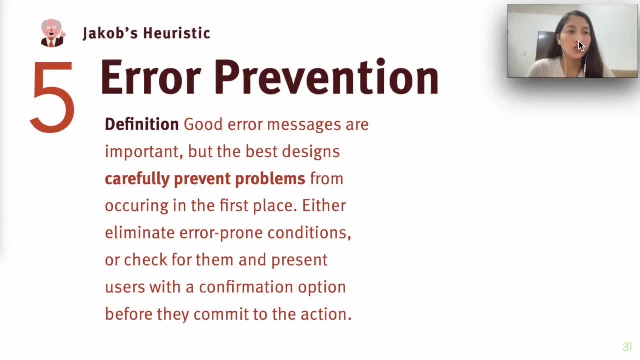 Okay. so if you avoid the mistakes of the users, that's the better option: either eliminate error prone conditions or check for them and present users with a confirmation option before they commit to the action. so here are some tips: prioritize your effort by preventing the high cost errors first, then little first. 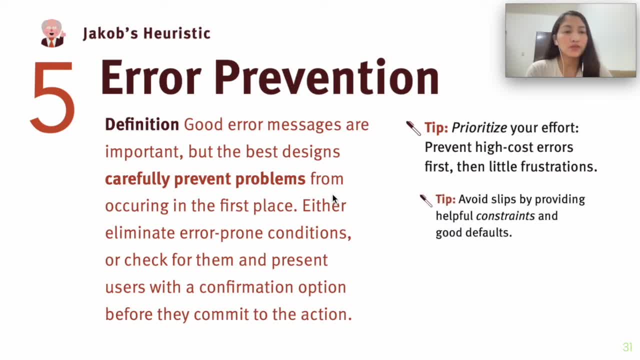 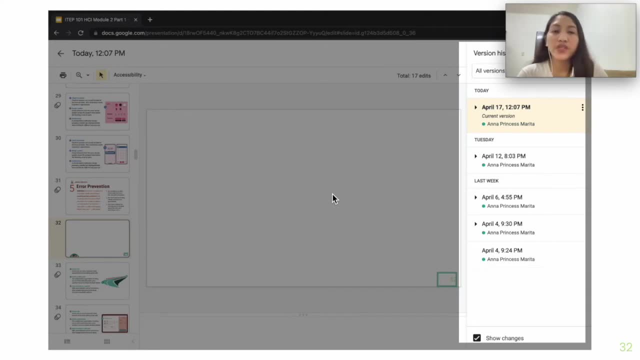 frustrations as you go along. second, avoid slips by providing helpful constraints and good defaults. and third, prevent mistakes by removing memory burden, supporting undo and winding your users. so this is an example in the Google slides, the version history feature of the Google slides, where you can restore the content of your slides, presentations or work to a state that is 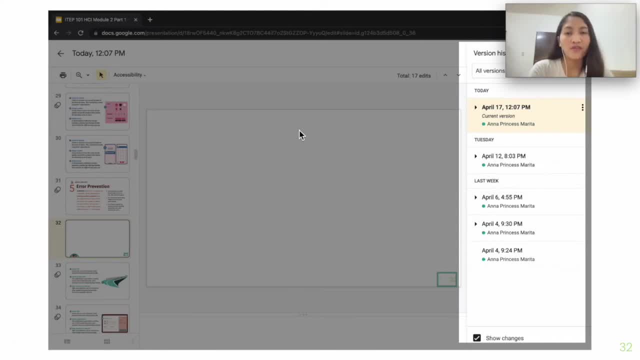 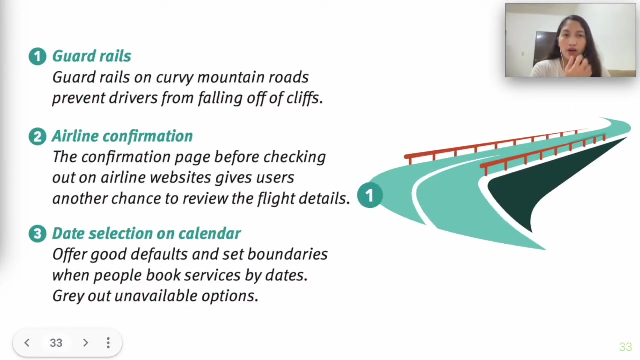 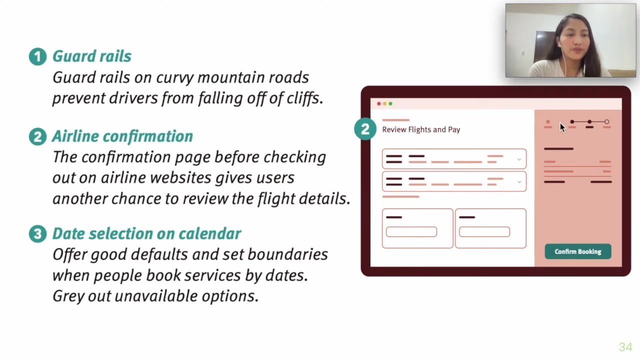 available here. so if you have inserted some things or some elements that are not supposed to be there, you can go back to the version of your choice. ok, so for the real-world example, we have the guardrails airline confirmation, the date selection on calendar. so let me discuss with you this airline confirmation where the user 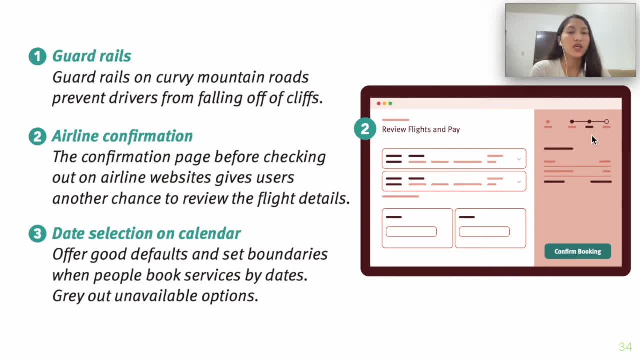 can review, or the customer can review the flight details before proceeding or confirming the booking, might know how his planeämä time and he is confident for for that person when he will be complete. so there should be a review of the flight alliances as well as the payment information information to the date selection on. 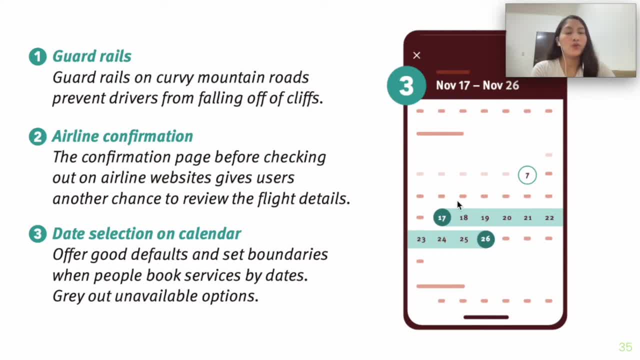 So ito naman halimbawa: magbubuk ka sa Airbnb, And if that date is not available for that specific accommodation, then it is disabled. If that is available, or that date is available or the dates are available, then you can click them. 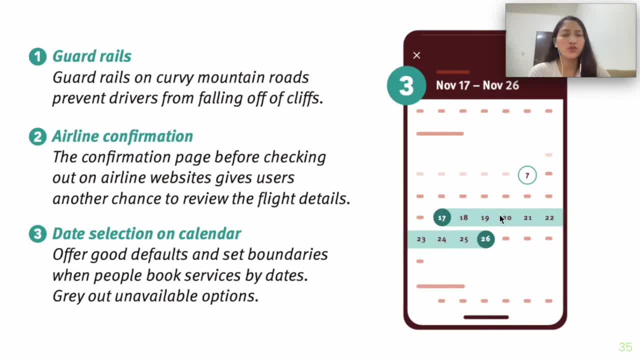 It is enabled. So to prevent, you know, double booking, triple booking and so on, Para ma-prevent yung mga bagay na yun. ay na-measure yung implication dun sa users mo. You really have to think through how to prevent errors. 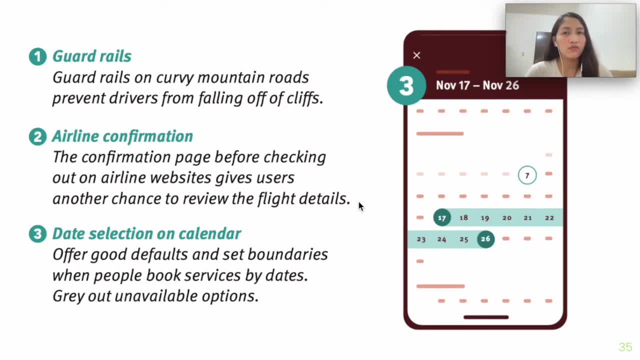 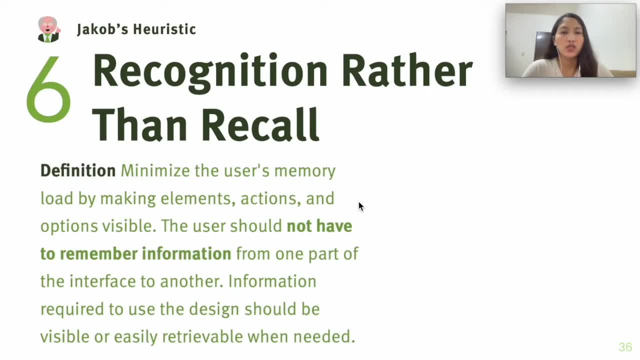 Because there are really systems na mahirap kapag nagkaroon ng errors along the way. Okay, so the sixth heuristic is recognition rather than recall. So you have to minimize the user's memory load by making elements, actions and options visible. 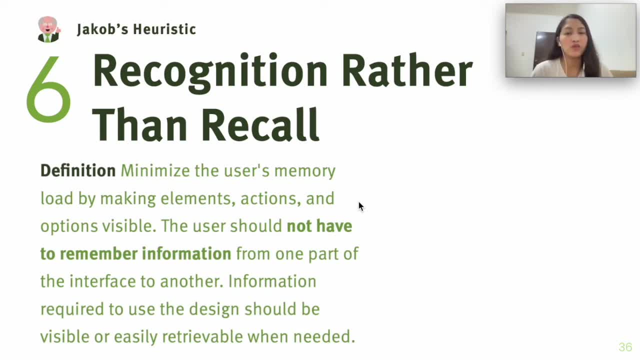 The user should not have to remember information from one part of the interface to another. Information required to use the design should be visible or easily retrievable when needed. So the first tip: let people recognize information in the interface rather than having to remember or recall it. 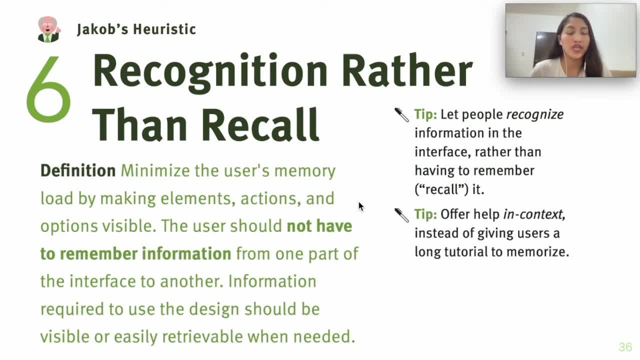 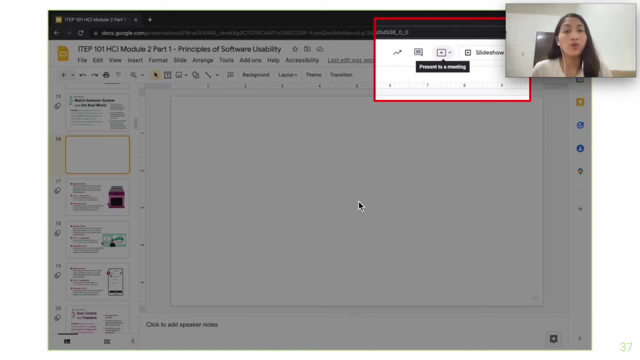 Okay, So we offer help in context instead of giving users a long tutorial to memorize and reduce the information that users have to remember. So let me go back to my previous example in the Google Slides, where, when you mouse over and information about a command or control button is being displayed. 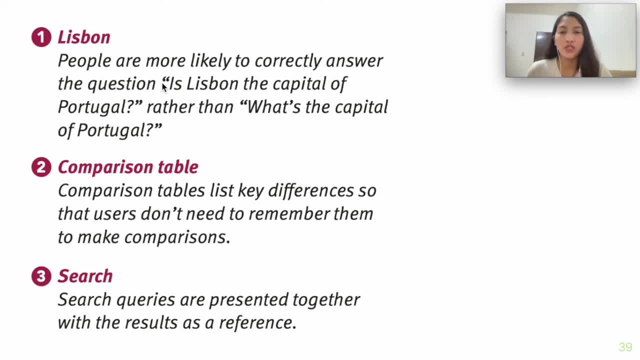 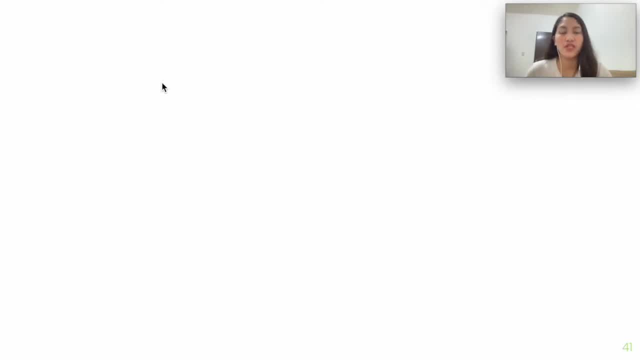 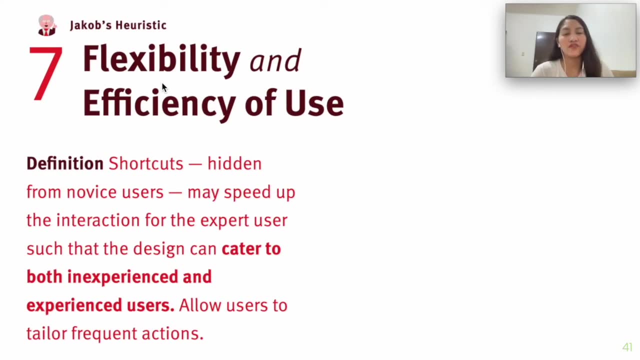 So here you have several examples: This one comparison table and the search. Okay, those are some of the implementations of this heuristic. The seventh is the flexibility and efficiency of use. We're talking about shortcuts here That's hidden from novice users. 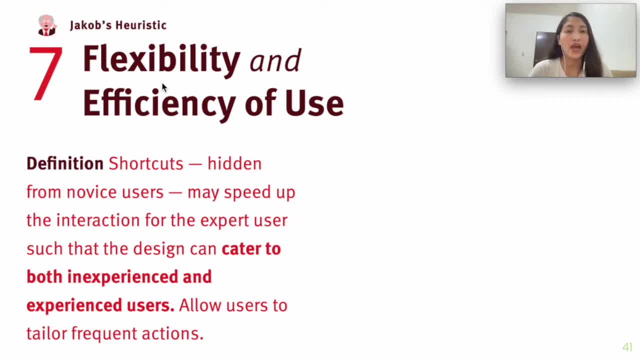 If you are new then probably you don't know the shortcuts of that specific app or system. But shortcuts may speed up the interaction for the expert users Right, Such that the design can cater to both inexperienced or experienced users. So allow users to tailor frequent actions. 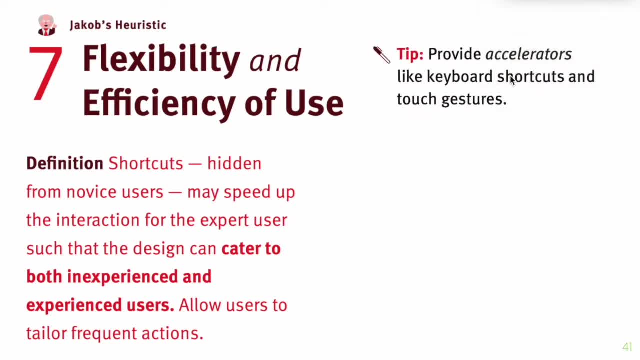 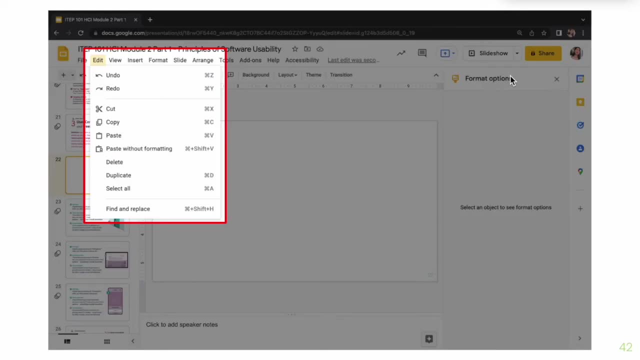 So the first step is to provide accelerators like keyboard shortcuts or touch gestures, Provide personalization by tailoring content and functionality for individual users and allow for customization. So you have here examples or an example in the Google Slide. Shortcuts are available, such as for the undo. 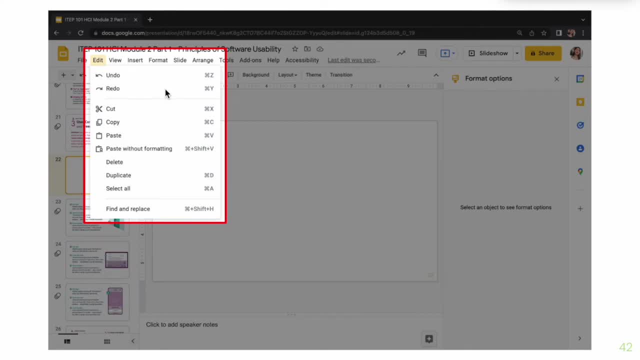 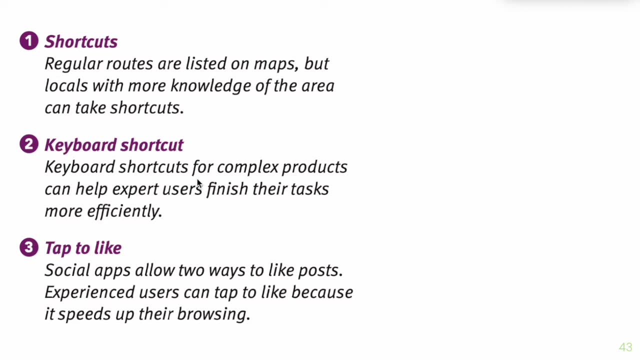 It is Command Z or Control Z for the Windows. So some of the real-world examples for this heuristic are shortcuts, the keyboard shortcuts and the tap the like. So instead of you know choosing options, you just have to tap it to like. 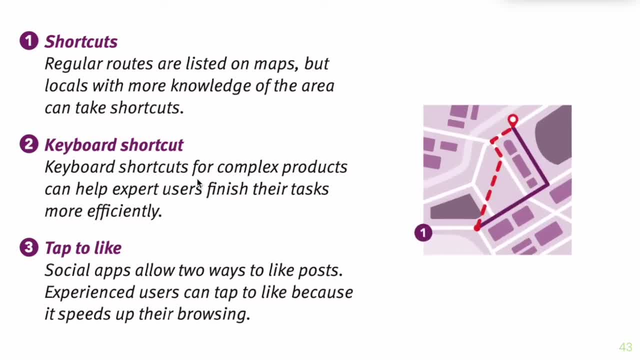 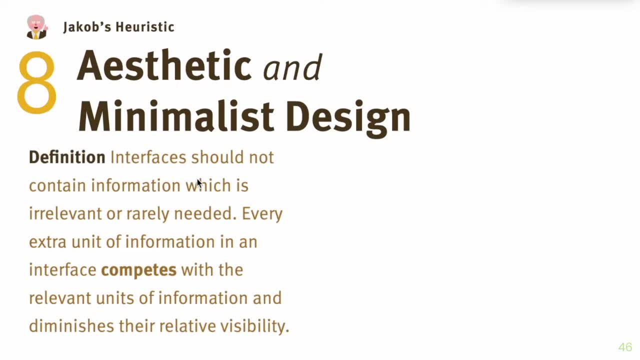 Just like in Instagram. So here: shortcuts, the keyboard shortcuts, and the tap the like. So the heuristic is the aesthetic and minimalist design. Interfaces should not contain information which is irrelevant and rarely needed. Every extra unit of information in an interface competes with the relevant units of information and diminishes their relative visibility. 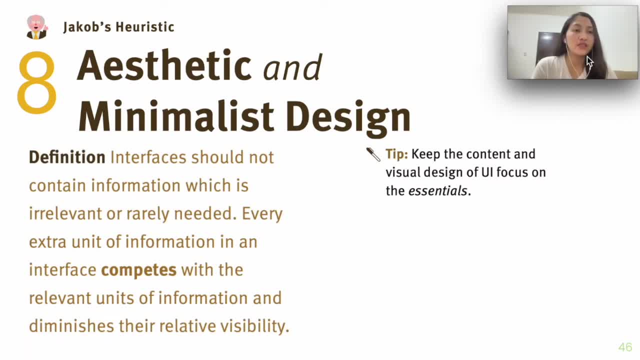 So the tips to apply this for implementation are the following: Keep the content And visual design of UI focus on the essentials. Second, don't let unnecessary elements distract users from the information they really need. And the third, prioritize the content and features to support primary goals. 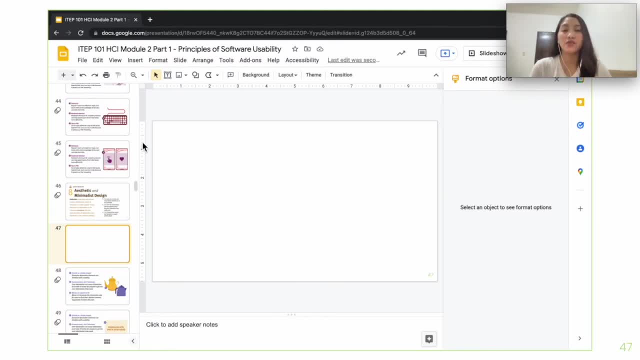 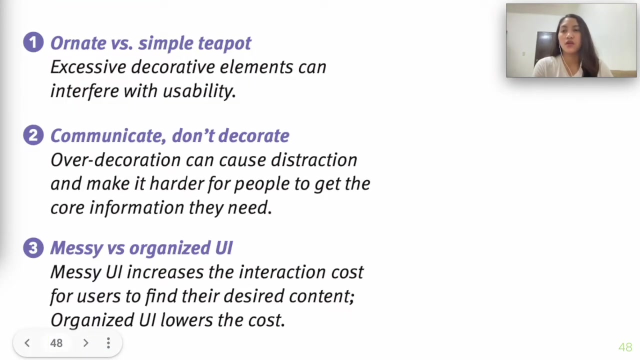 So an example is again the Google Slides, where you show the options That are available or that can be done when you are clicking or you are working on an element in your presentation. Okay, so the next is some more. examples are the following: are Nate versus Simple Teapot? 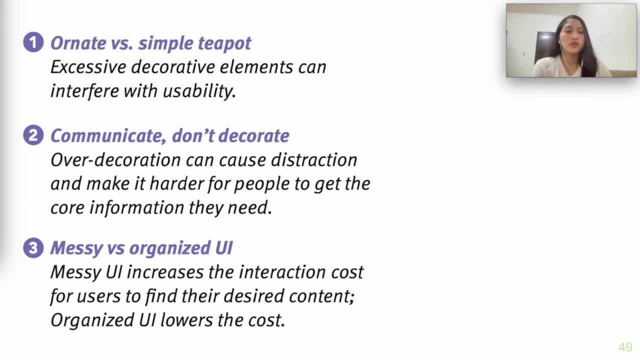 Communicate, don't decorate. So communication is different than Decoration. sometimes an interface is over-decorated- masyado na siyang, madaming design, over-designed na siya okay, And nawawala na yung usability, yung efficiency ng use and the messy versus organized UI. 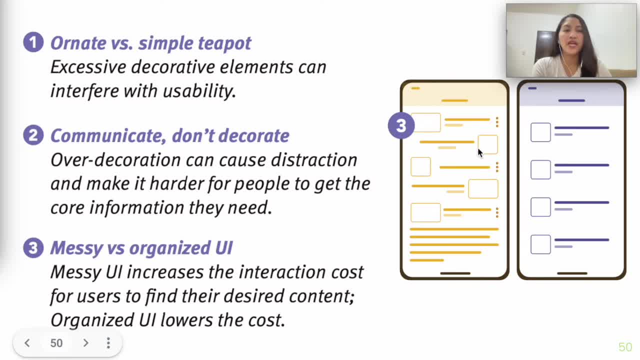 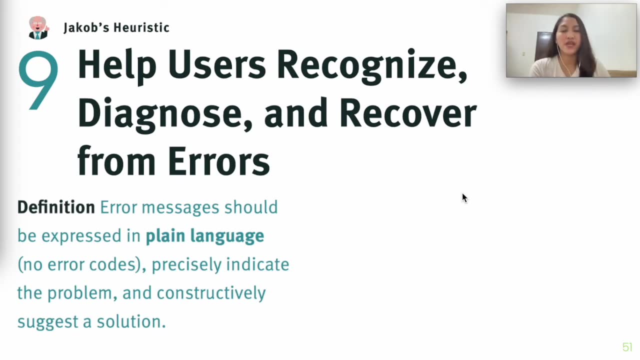 So you really have to work on that. So you really have to work on that. So you really have to work on that. So you really have to work on making an organized UI rather than a messy one. Okay, so the ninth heuristic is the help users recognize, diagnose and recover from errors. 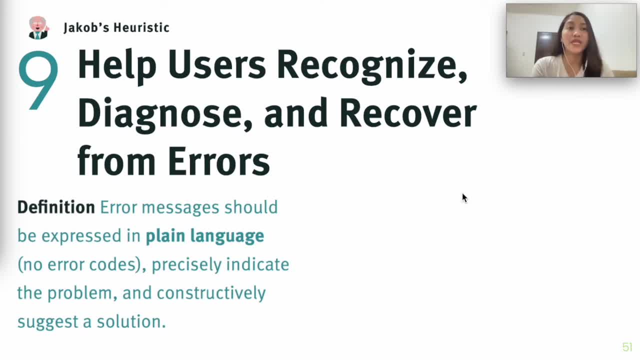 So error messages should be expressed in plain language. No error codes Precisely indicate the problem and constructively suggest a solution. So the tips are: use traditional error messages message visuals like bold red text. but these are some conventions that you can tweak according to the design standards or design conventions that you are applying in your design. 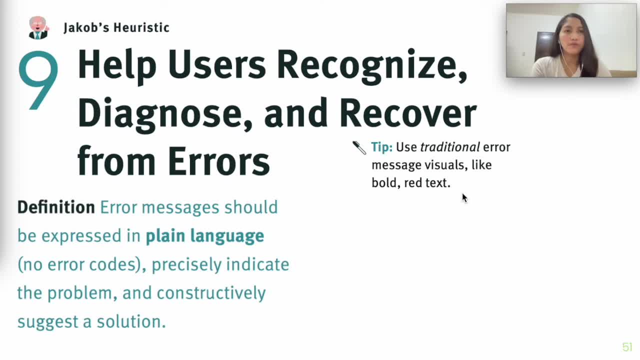 Pwede hindi naka-red text, pero yung design ng error message ay. alam mo lang na the user has created a message. Pwede hindi naka-red text, pero yung design ng error message ay. alam mo lang na the user has created a message. 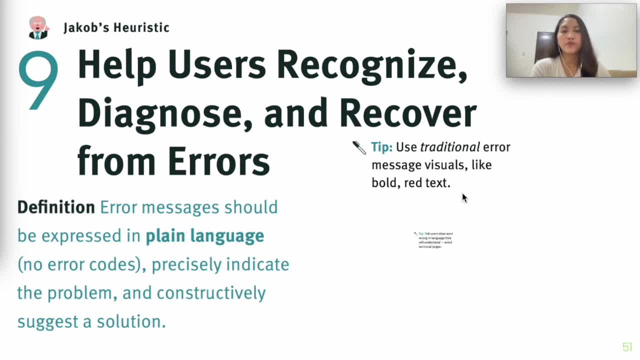 So if you make a mistake, by accident or not, Tell users what went wrong in language that they will understand. Avoid technical jargons such as error 101 or code 502, error, something like that. So tell them in the language that they can understand. 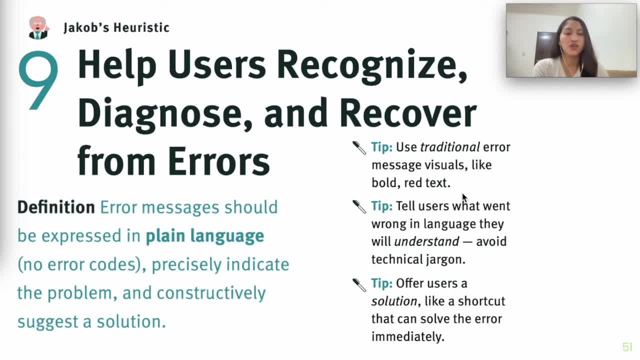 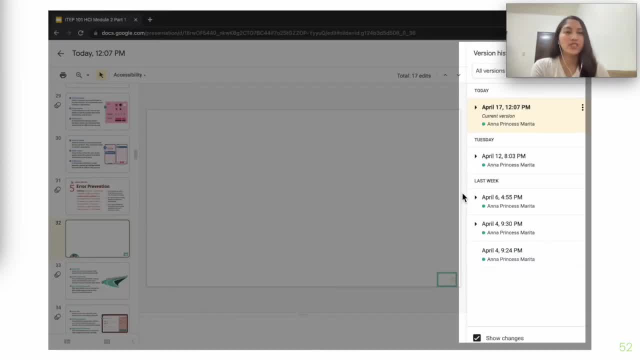 And then offer users a solution like a shortcut that can solve the error immediately. So tell them in the language that they can understand, And then offer users a solution like a shortcut that can solve the error immediately. So I will just show you this as an example implementation for that heuristic. 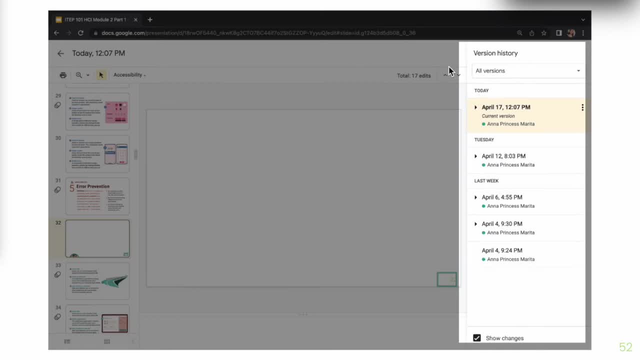 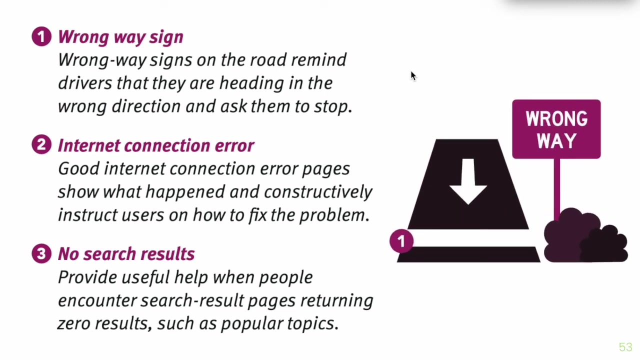 Okay, but there are different implementations of that heuristic of displaying the error messages and actions for an error message. Okay, so you have here real-world examples: the wrong way sign, So the wrong way. signs on the road remind drivers that they are heading in the wrong direction and ask them to stop. 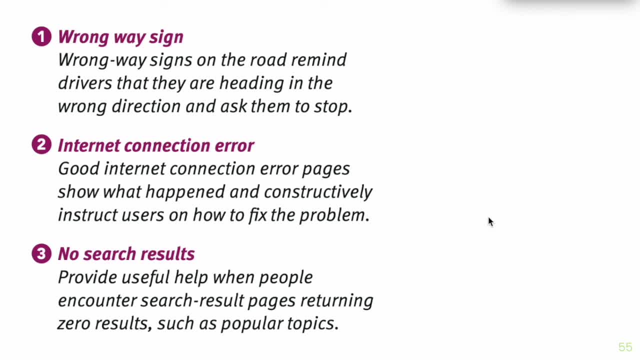 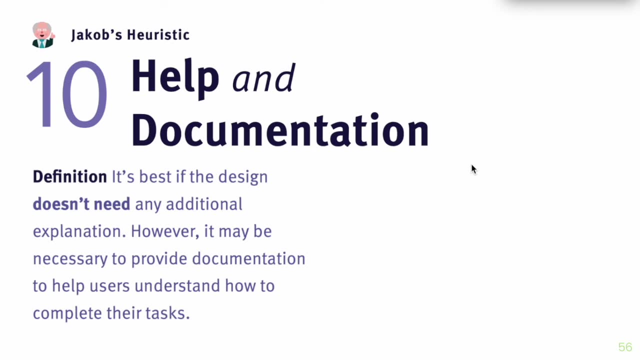 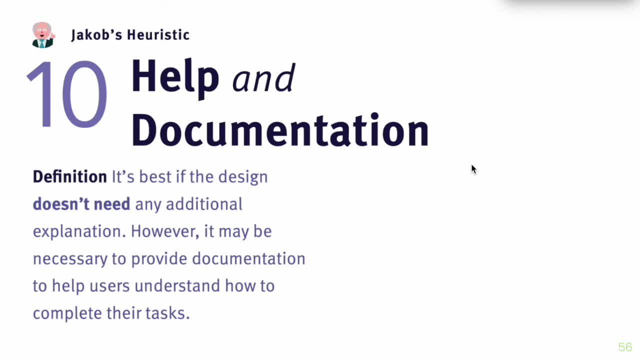 It's best if the design doesn't need any additional explanation. However, it may be necessary to provide documentation to help users understand how to complete their task. So some tips: Ensure that the help documentation is easy to search Whenever possible. present the documentation in context right at the moment that the user requires it. 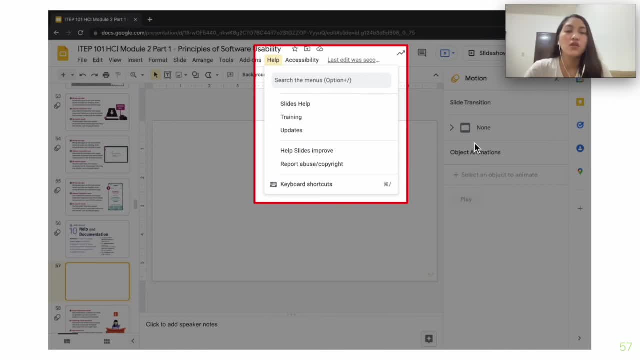 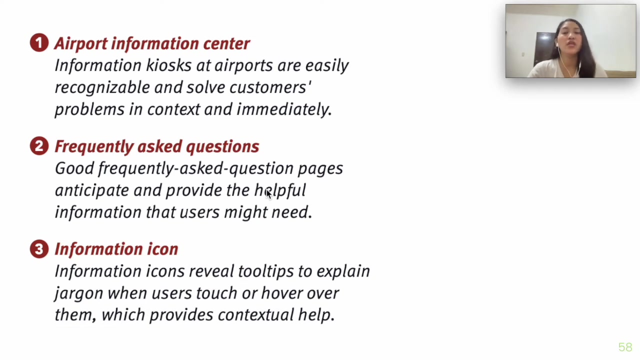 And then list concrete steps to be carried. So in Google Slides you also have the help options and the mostly searched things in the help. So the real-world examples are the following: Airport Information Center. So it's easily recognizable to solve customers' problems in context and immediately. 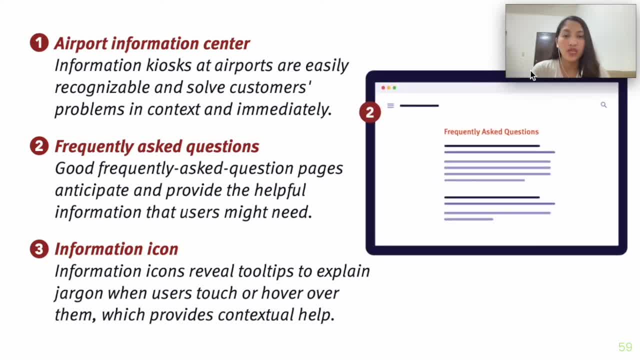 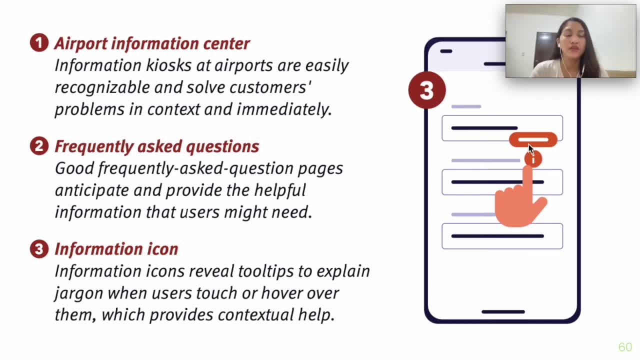 So it's easily recognizable to solve customers' problems in context and immediately: The Frequently Asked Questions page And the information icon where you can tap it in order for you to know what's going on, More details about that specific thing that you want your users to know, or the information that is being shown to them. 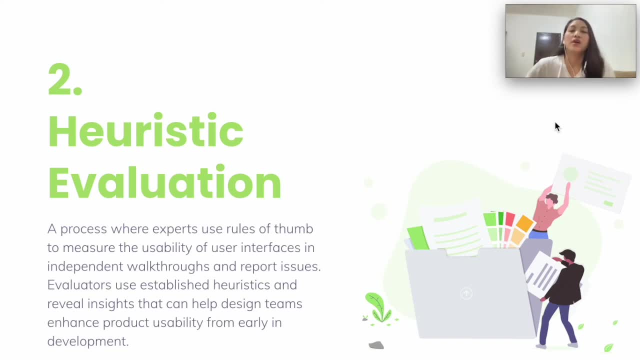 Next we have the heuristic evaluation. Heuristic evaluation is a process where experts use resources. It's a rule of thumb to measure the usability of user interfaces. in independent walkthroughs and report issues, Evaluators use established heuristics, just like the Jacob Nielsen's heuristics, and reveal insights that can help design teams enhance product usability from early in development. 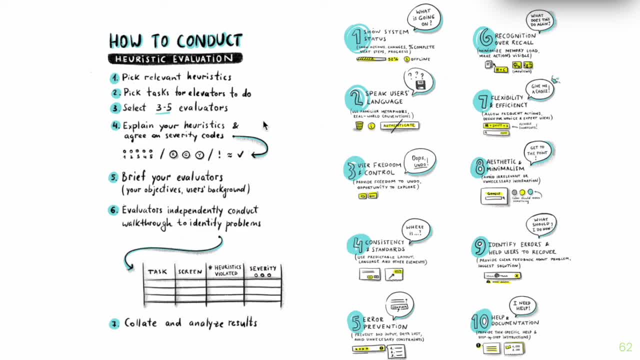 So how do you conduct that? So you have here, Of course, you have your heuristic, So you have your heuristic ready at hand, And then these are the steps. We have seven steps. So the first one: pick relevant heuristics. 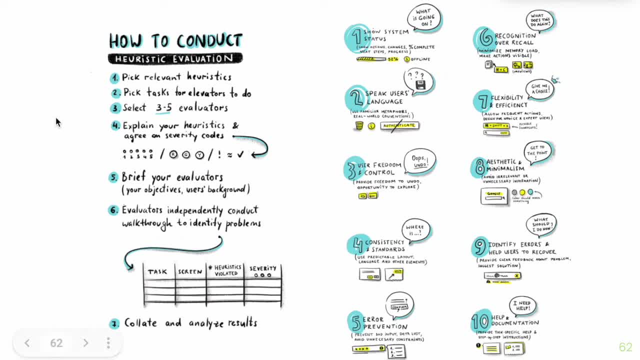 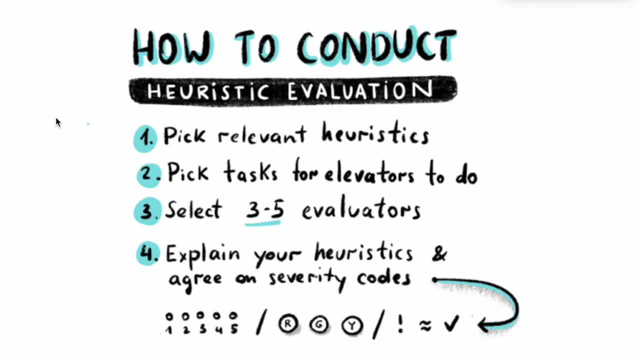 So in this case you have picked the Jacob Nielsen's heuristics, But you can also use other heuristics that are available And then pick tasks for evaluators to do. Evaluators don't know. Pick tasks for evaluators to do. 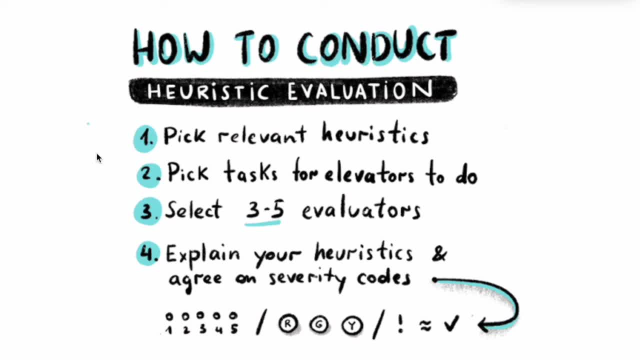 And then select three tasks. So you have three to five evaluators. Why three to five? Because if it's just one, the errors that you will see or the improvements that you will see are limited, as compared to if there are three or five of you who are looking for, analyzing or evaluating the user interface. 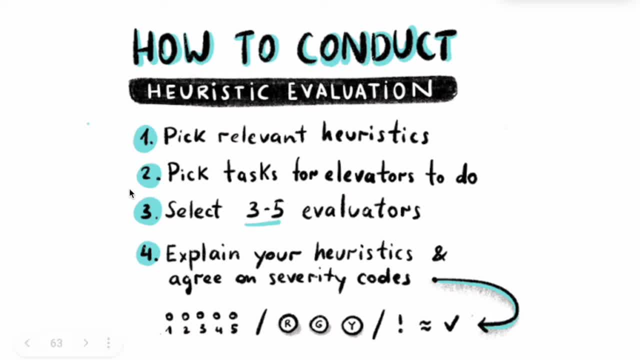 And then explain your heuristics and agree on severity codes. For example, this heuristic: you may have seen an error, But its severity is the same. It's from one to five, Five being the highest. Or it can also be that it requires immediate action. 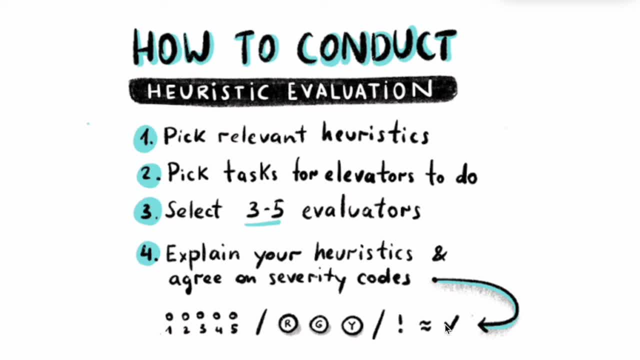 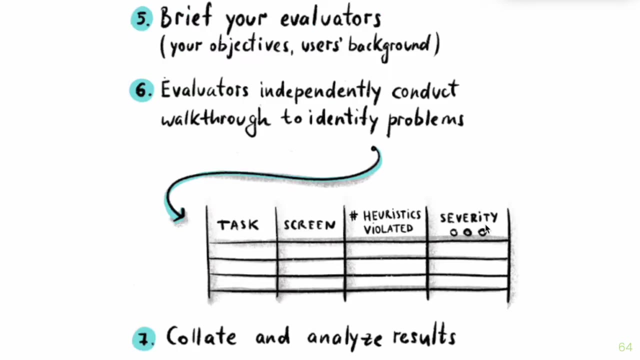 This is neutral, The other one is agreeable or okay. The specific feature or heuristic is okay for the whole user information. And, by the way, you have to assign UI parts for each evaluator, So you have to brief your evaluators about your objectives, the user backgrounds, the user interface sequence and the evaluator's independently conduct walkthrough. 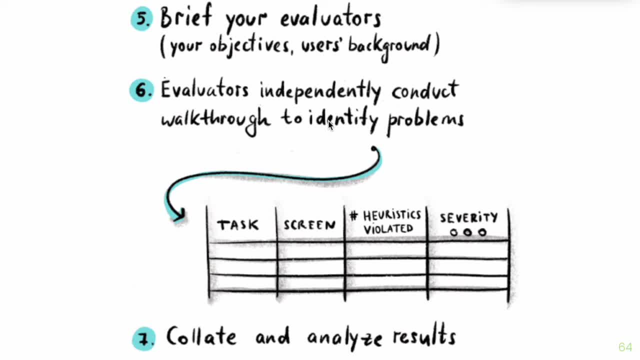 So they are independent. They are one by one. Probably they are not together, But they can be together. But they have their own thing. It depends on what is assigned to them as UI parts, Or what is assigned to them as UI parts. 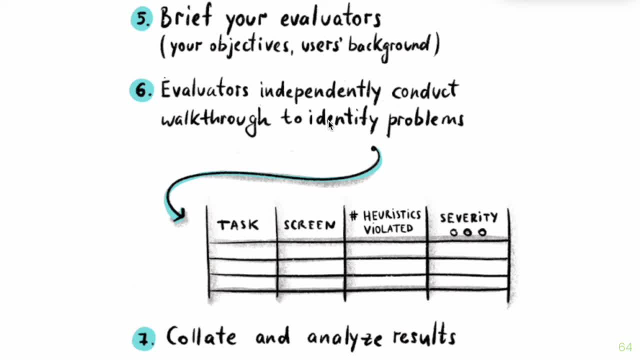 Or what is evaluated on their user interface. So you have to, Then the evaluators can. You can use a form in order for the evaluators to write on. So here they have used this form including the task, the specific task, the screen, the heuristics that are violated. 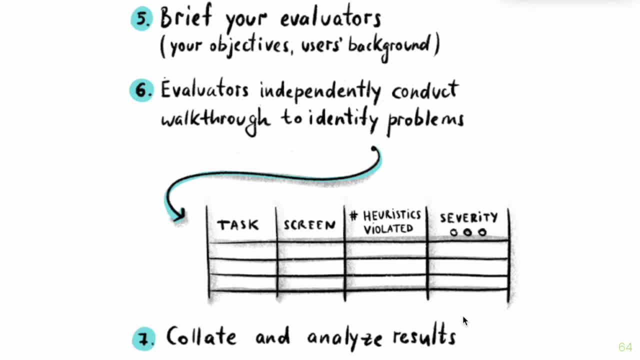 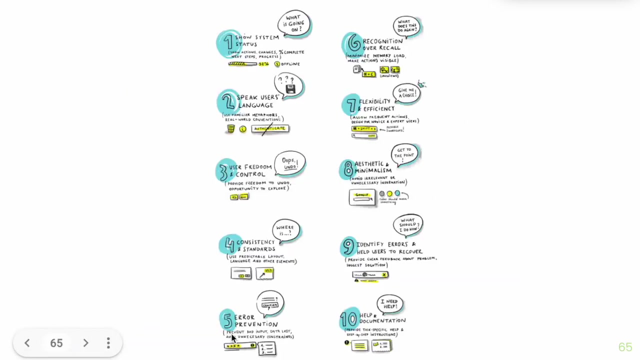 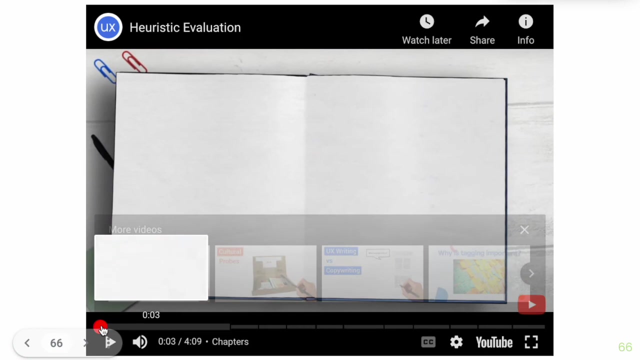 And the severity here on this column. okay, so, and then after that, after they have conducted a walkthrough to identify the problems for the whole user interface or for the different parts assigned to them, then that's the time that you can collate and analyze the results. so this, so this is a video about the heuristic evaluation. so 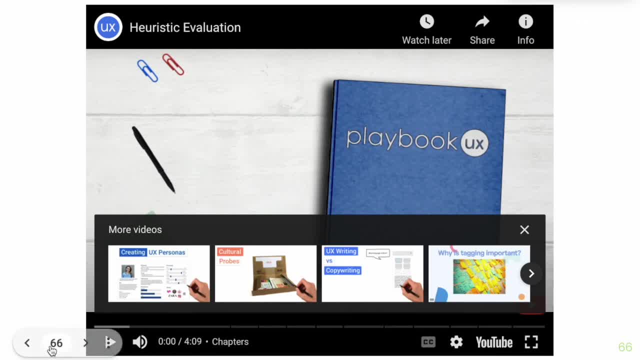 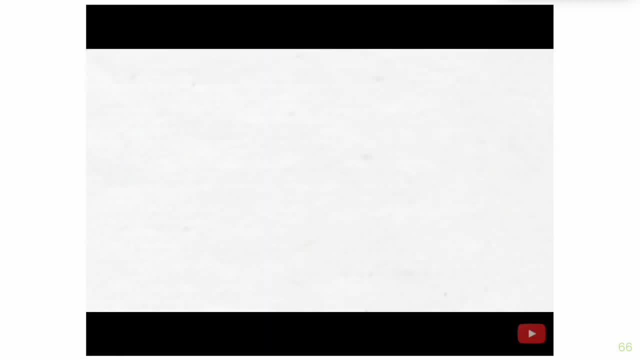 let's all watch this video. in this video, we'll walk through heuristic evaluations. a heuristic evaluation, also known as an expert review, is a way to ensure your website is user-friendly. a heuristic evaluation is similar to user testing, but in user testing the testers are users and heuristic evaluations the. 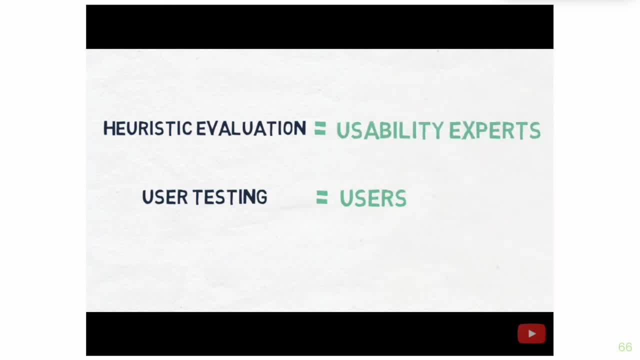 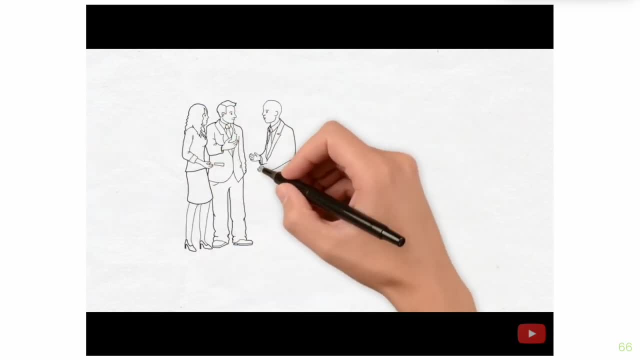 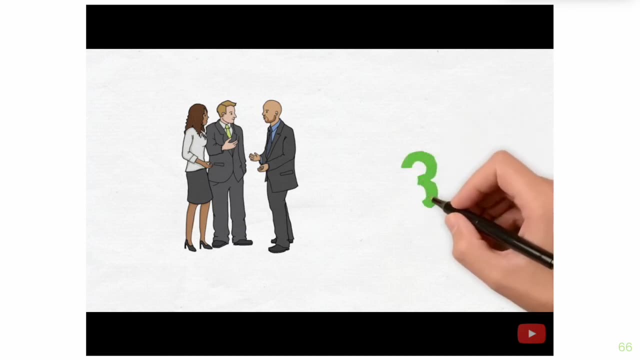 testers are usability experts. heuristic evaluations should be conducted alongside user testing early on in the software development lifecycle. these usability experts are professionals who are skilled in determining heuristic evaluation criteria and assessing a product against it. it is recommended that three usability professionals independently assess your product. however, startups can't always afford to hire three usability experts, so you can. 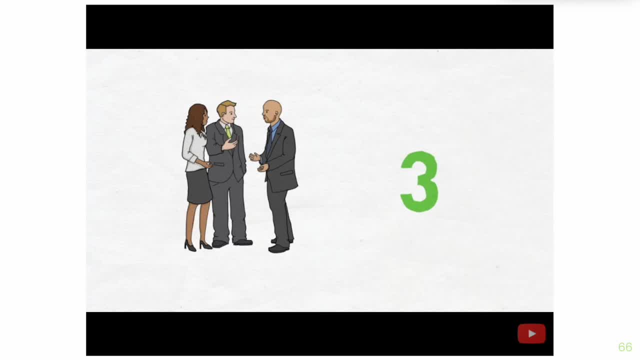 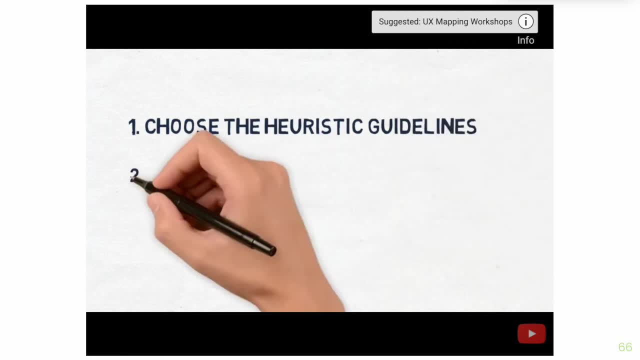 perform what's called the heuristic markup, which is where you perform the assessment yourself. in order to perform a heuristic evaluation, the usability experts must first choose the heuristic guidelines, second, define a rating system and third, choose a method for documentation. there's a list of 250 plus qualitative guidelines to test against. however, it's safe to use Jacob. 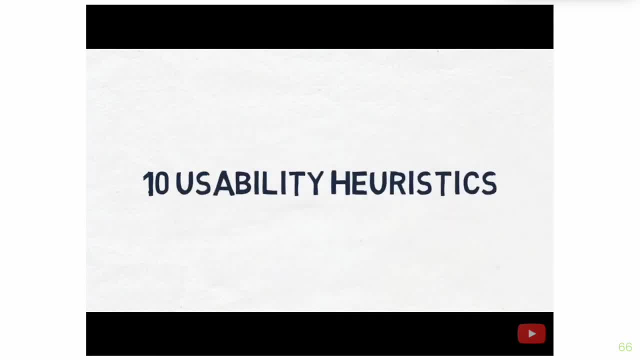 Nielsen's ten usability heuristics. as a starting point, we'll walk through some examples of the good and the bad. first, there's visibility of a system status. the system should keep users informed of what's going on. in this example, tiny PNG shows you that there are three PNGs that have been 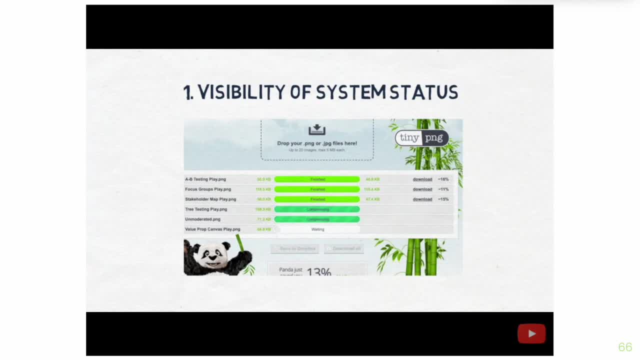 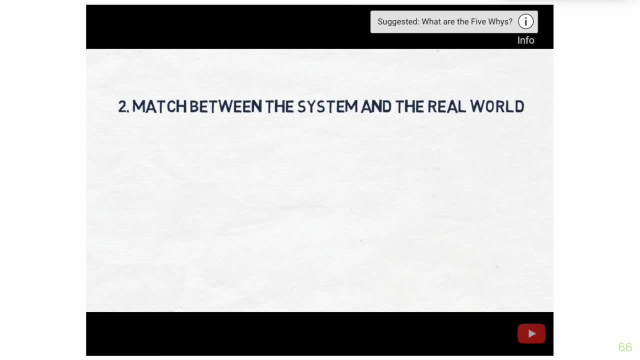 compressed, while two are in progress and one has not started yet, match between the system and the real world. the system should use language that is easy for your target user to understand. this is extremely important for error messages. in the below example, Microsoft produces an error. the human simply cannot. 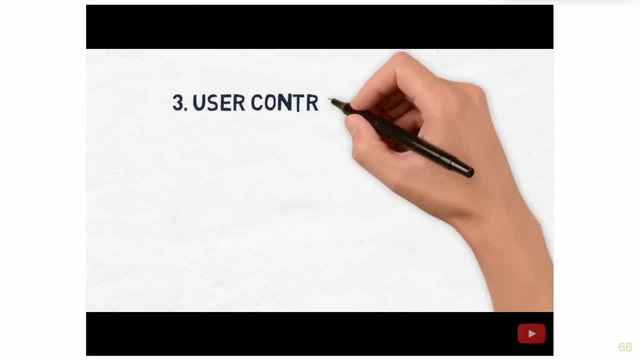 understand. third, user control and freedom. users should be able to undo and redo actions and also have the ability to move backward. there should always be an emergency exit. Gmail allows you to undo actions. this is important, since people make mistakes. fourth, consistency and standards. screen elements should be consistent across the entire platform. Microsoft's header bars. 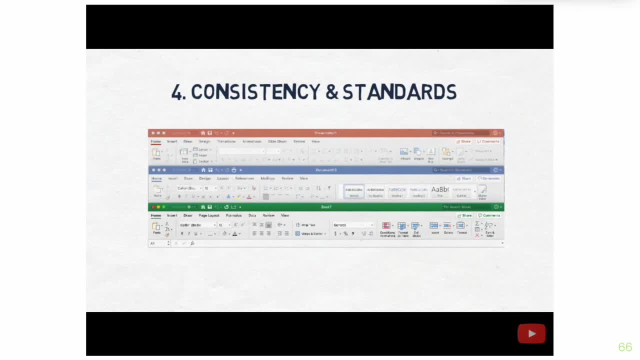 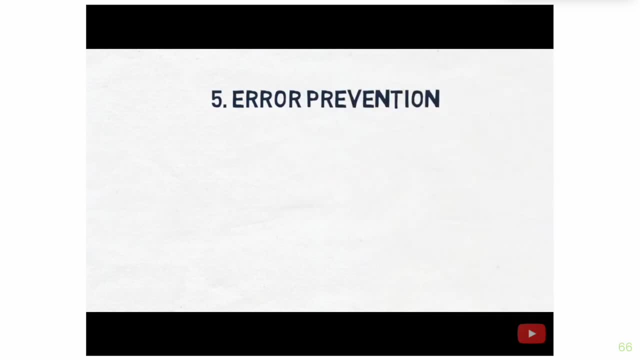 are identical for Word, Excel and PowerPoint, so users can switch between the three applications seamlessly. fifth, error prevention. error should be kept to a minimum. you should try and prevent errors from happening by crafting careful design so users can't break your system. in this example, Gmail tries to limit your errors when you write- see attached in an email. 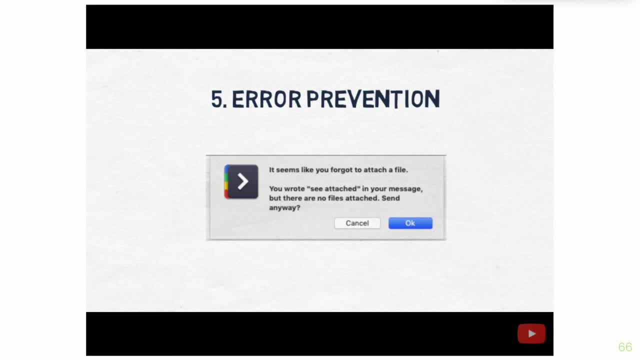 Gmail checks to see if you have an attachment, to make sure you didn't forget to attach a document. recognition rather than recall minimize the user's cognitive load by making information from one part of the website relevant to another part of the website. when you visit Amazon, they include a list of your 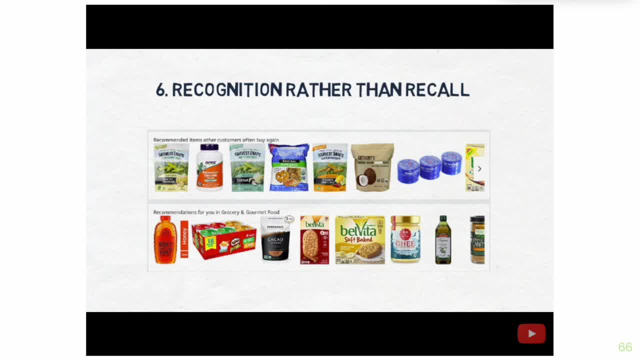 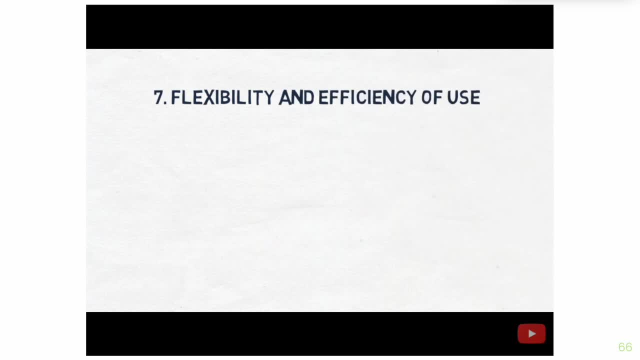 recently viewed items and they provide suggestions based on your past searches. seventh, flexibility and efficiency of use. shortcuts allow experts to speed up the experience while being unseen to the novice user. these shortcuts are important because your system should cater to all ranges of expertise. in this example, Google hides the advanced features under more 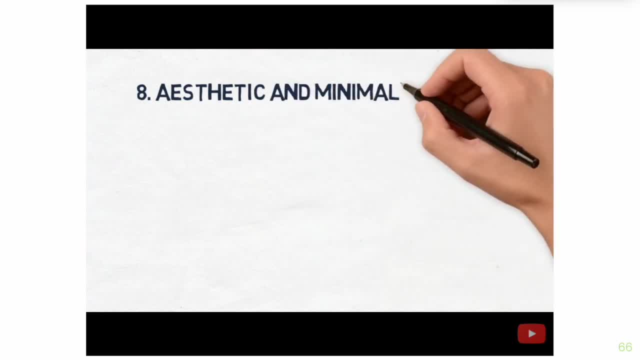 aesthetic and minimalist design. irrelevant information should not be included in your design. you should limit the design to must have elements only. Google landing pages are very simplistic and easy to navigate. ninth, help users recognize, diagnose and recover from errors. error messages should use plain language without codes. it should indicate the problem and suggest. 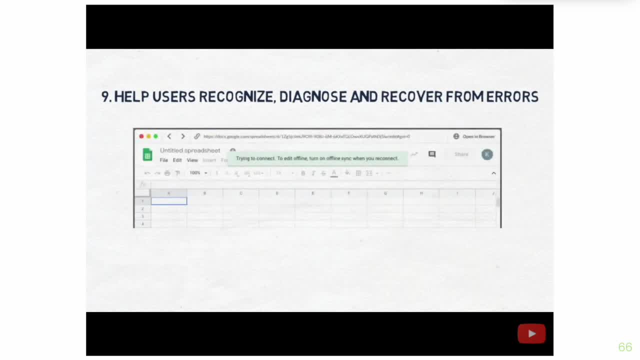 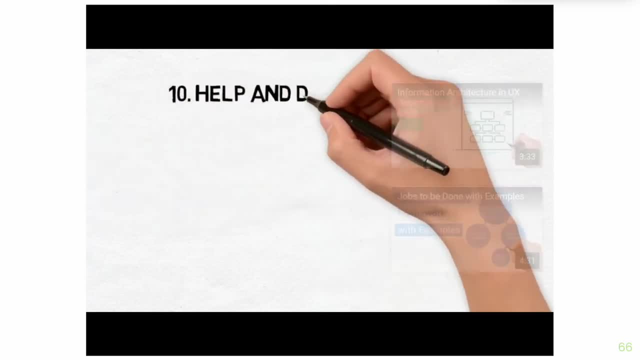 a solution since I'm offline. Google sheets lets me know that's why I can't edit my document and provides a solution to prevent this error in the future. lastly, help and documentation. although the ideal system shouldn't need documentation, there still should be documentation to provide the user. 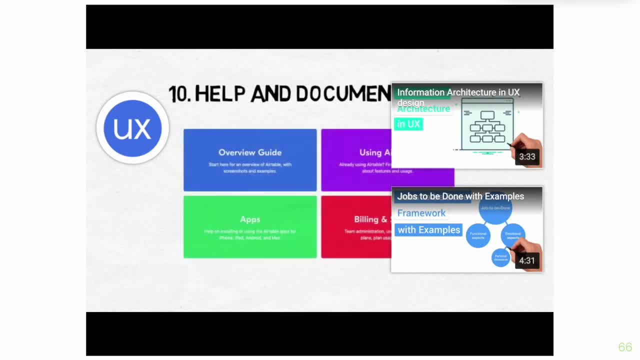 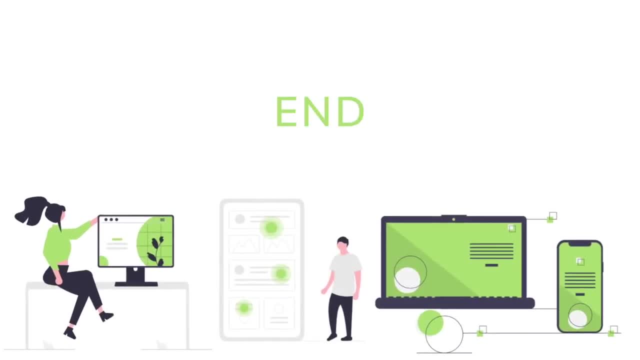 with additional information air table- just a documentation so they can find answers on the fly. thanks for watching you.